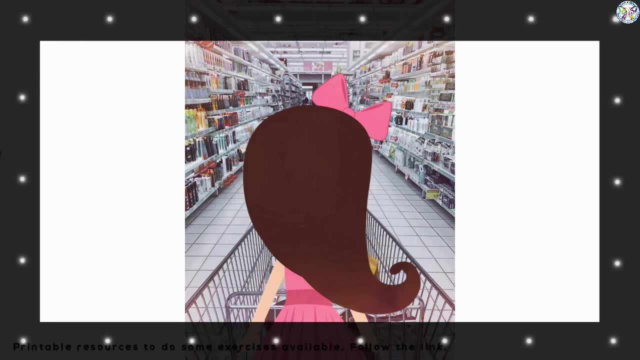 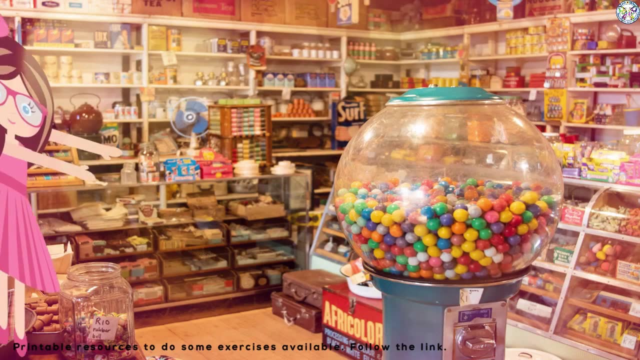 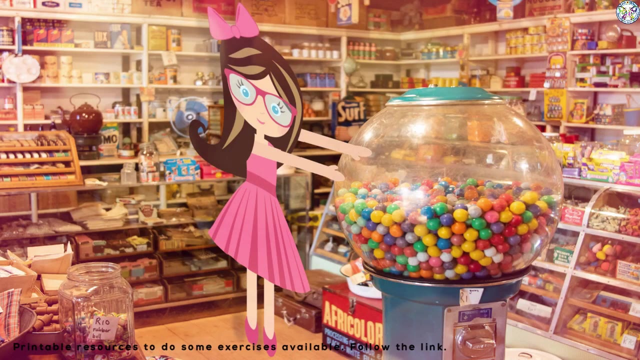 this. I bought her a sandwich. Yeah, what do you want? And what do you want of shops? let's go along with Emma, mmm. a sweet shop. I love sweets and you. Emma looks around and chooses one of the sweets. she takes out of her purse: a five. 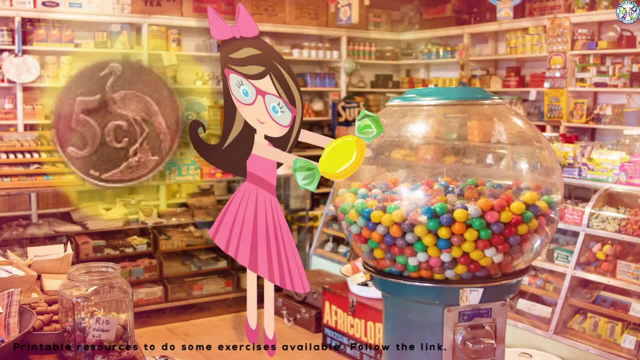 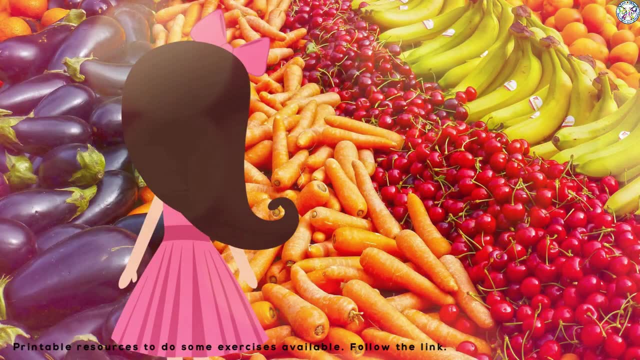 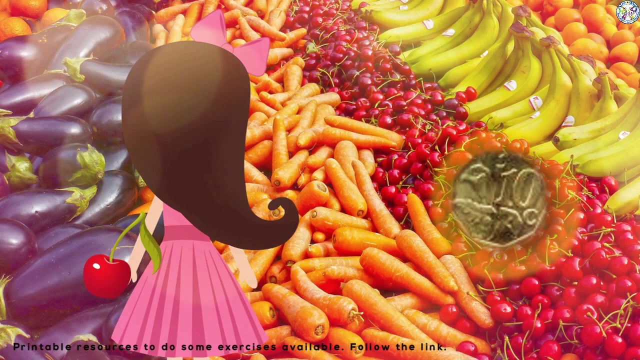 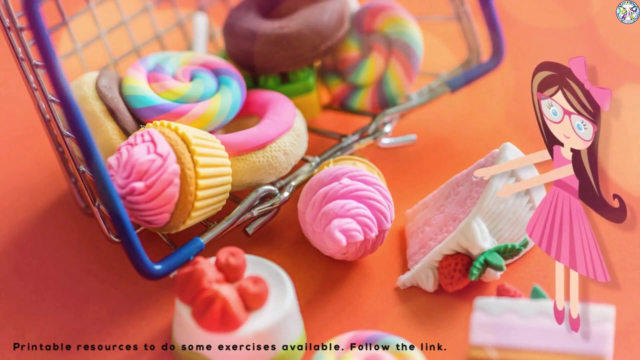 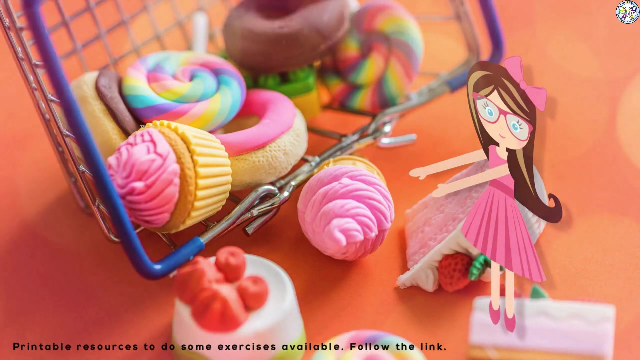 cent coin and pays with it. an excellent choice. the green grocer, Emma, looks around and she chooses a yummy red cherry. she takes out of her purse a 10 cent coin and pays with it. it is a French birthday tomorrow and she wants to take along a delicious piece of cake. yummy, a. 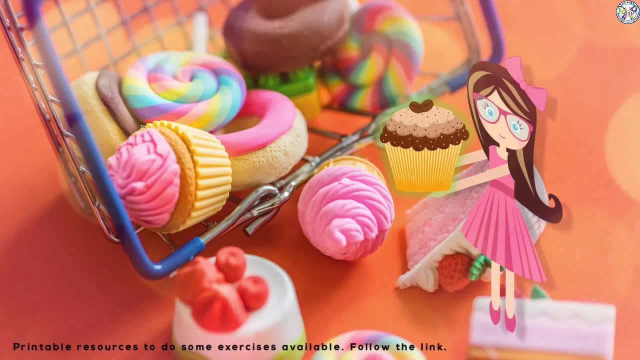 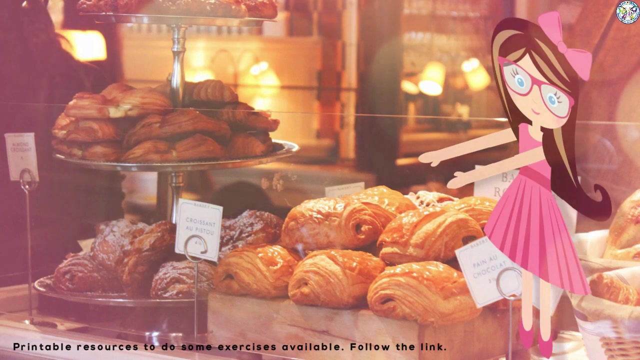 chocolate cake. what a brilliant choice. she pays for it 20 cents and off she goes to the next shop- the bakery- there's loads of nice stuff. she prefers a chocolate cake. and she takes out a 20 cent coin and off she goes to the next shop- the bakery- there's loads of nice stuff she prefers. 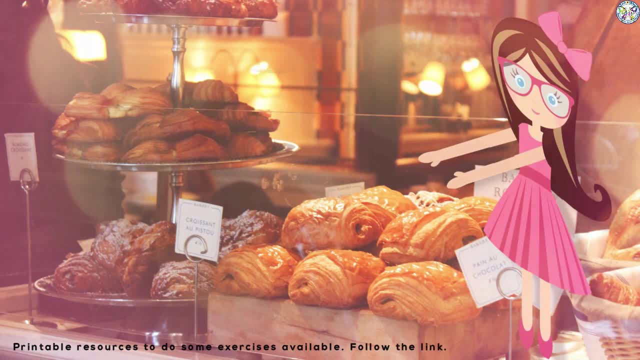 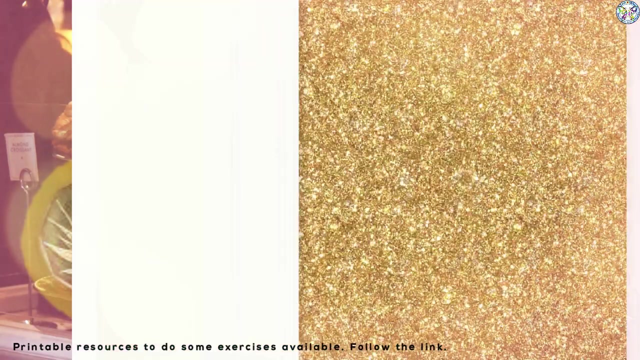 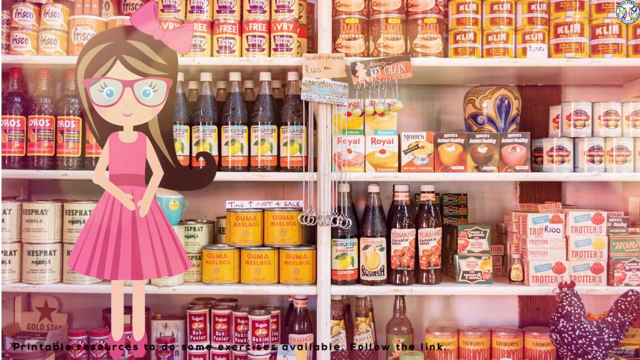 a healthy bread to make herself a sandwich, maybe a hamburger for a lunch for the afternoon. she pays 50 cents for the bread to make herself a sandwich off. she goes to the supermarket again. she wants to put some pineapples on her hamburger roll. she chooses a tin of. 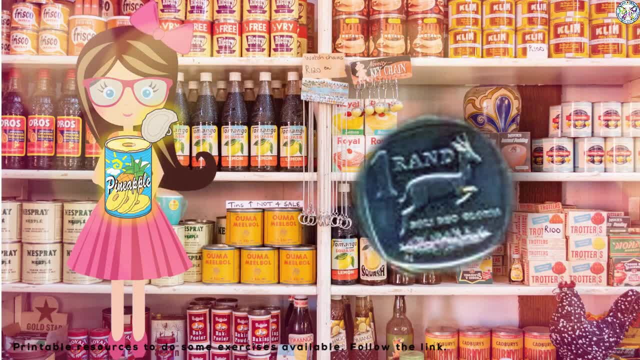 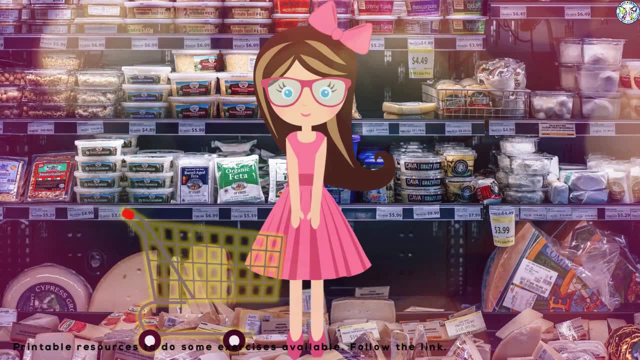 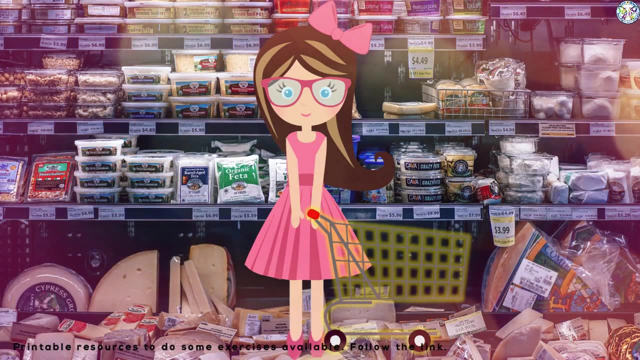 pineapples and she pays one Rand to the lady behind the till. she takes a trolley and makes a turn at the aisle with all the different cheeses. she decides on the yummiest cheese of all and then she has to pay for it. 100 Sure videos Sur exclusively on Smaragamcom. 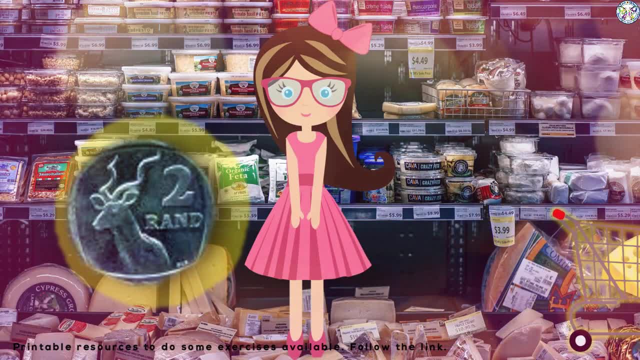 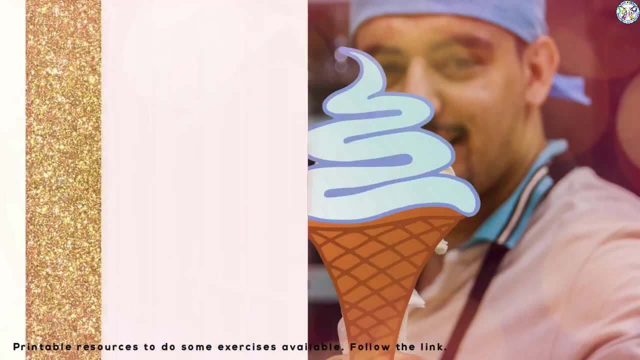 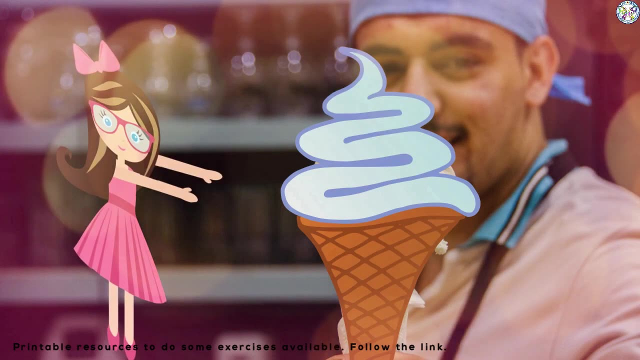 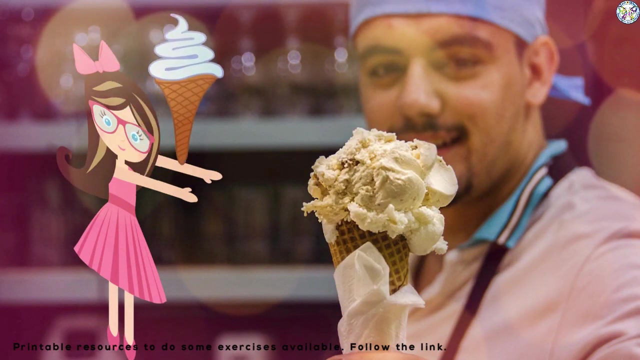 She pushes a trolley out and pays with a two rand coin. It is very hard work to do shopping. She decides to treat herself with an ice cream. She takes the ice cream cone from the man who smiles back at her when she gave him a. 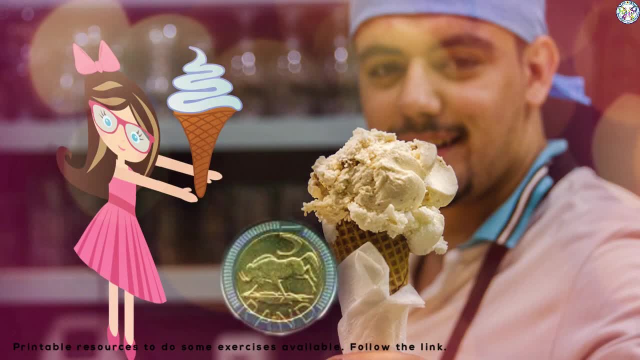 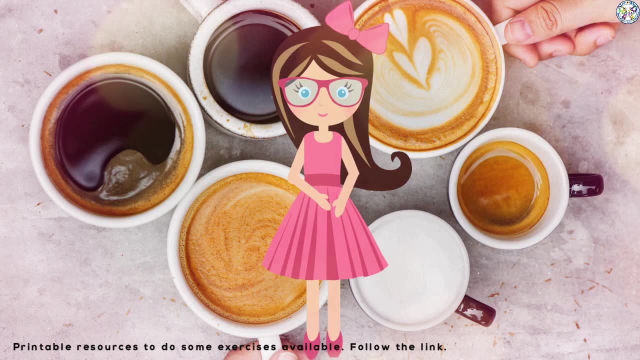 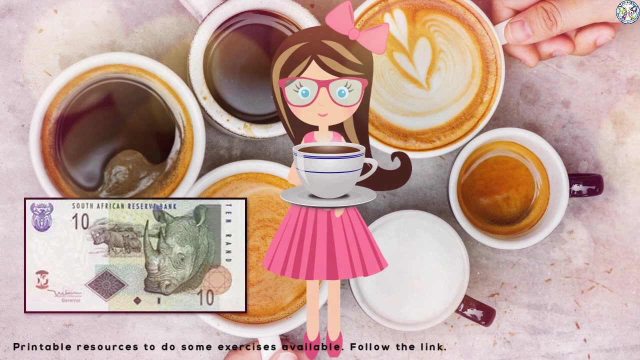 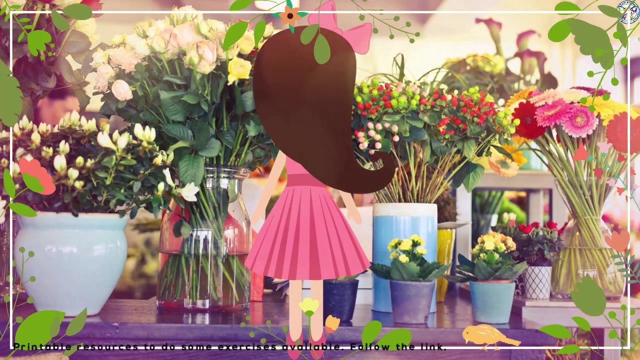 five rand coin. Emma needs some coffee, so she decides to go to the coffee shop where she buys herself a hot, steamy cup of coffee. That cup of coffee costs her ten rand. She pays with a ten rand note. Emma wants to buy her mum a bunch of flowers. 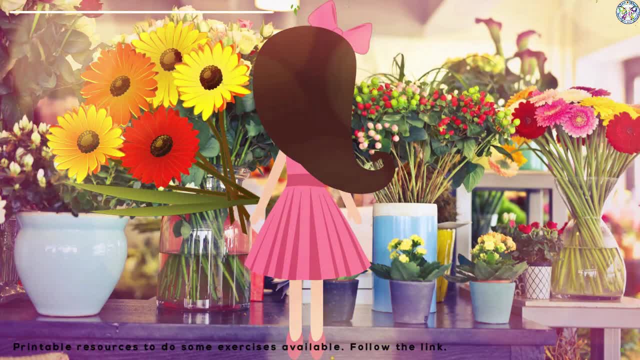 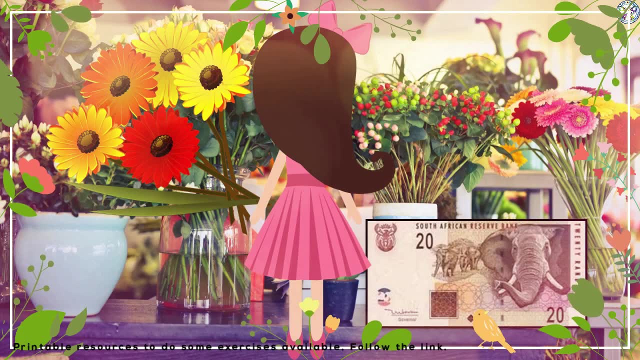 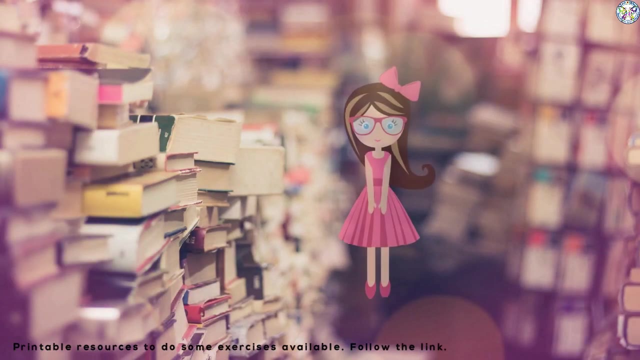 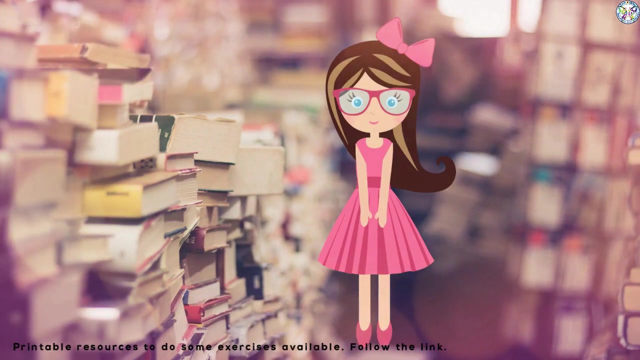 She picks up a colourful bunch of flowers and that bunch of flowers costs her twenty rand. She pays with a twenty rand note. She cannot survive without reading a very good book. She walks in the bookshop and picks a very nice novel. She looks in the novel and sees the price. 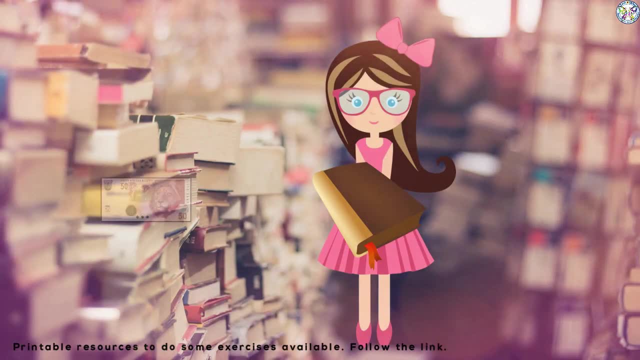 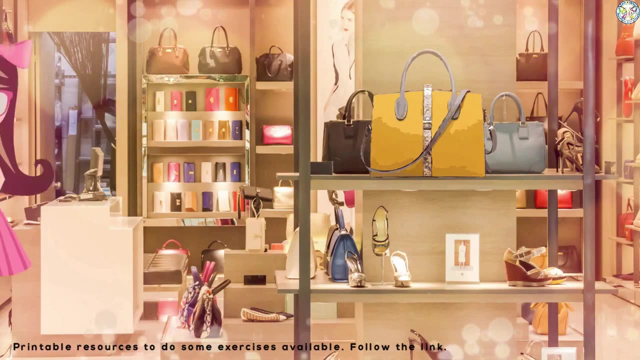 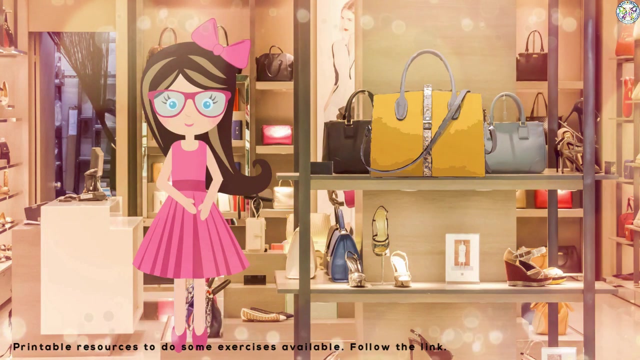 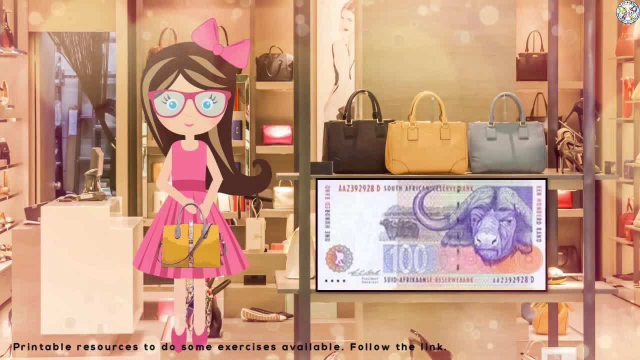 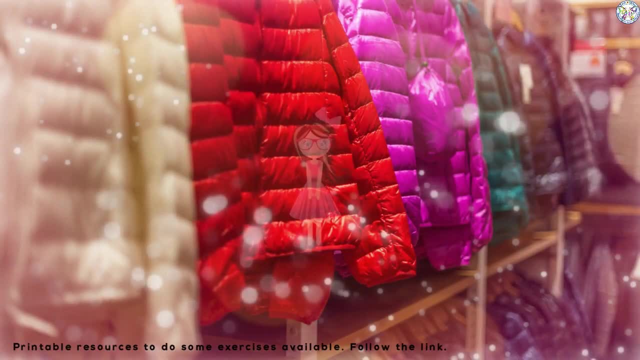 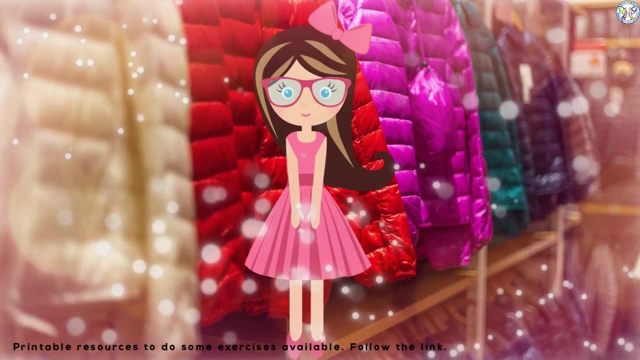 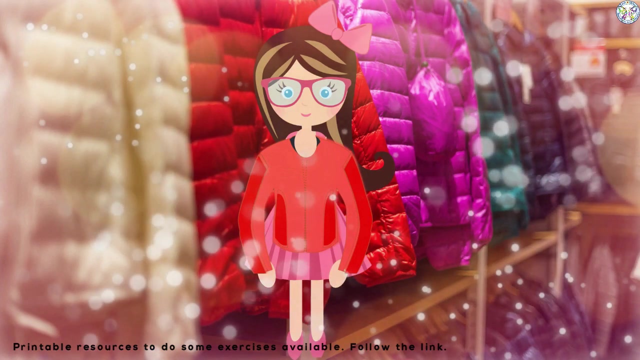 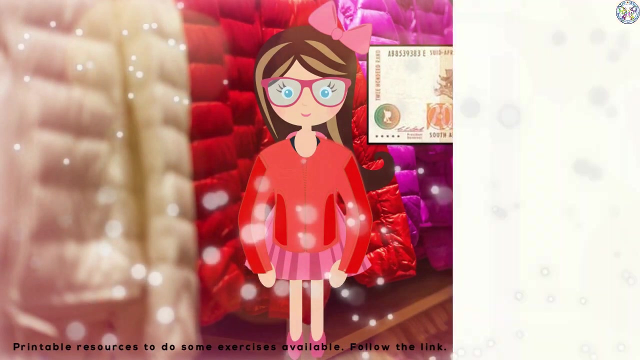 She needs to pay with a hundred rand bank note. A nice colourful jacket for the upcoming winter? What about a red one? A red one? It is a bit expensive. She knows It will last her a lifetime. She pays with a 200 rand note. 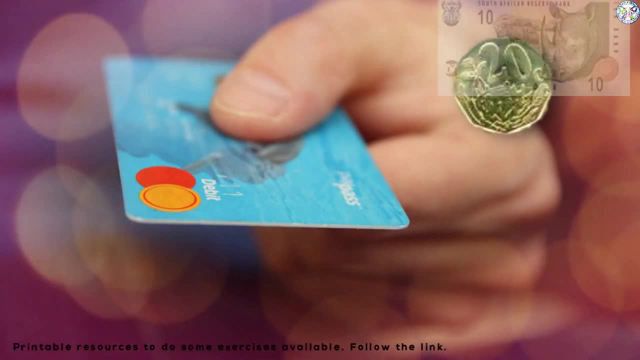 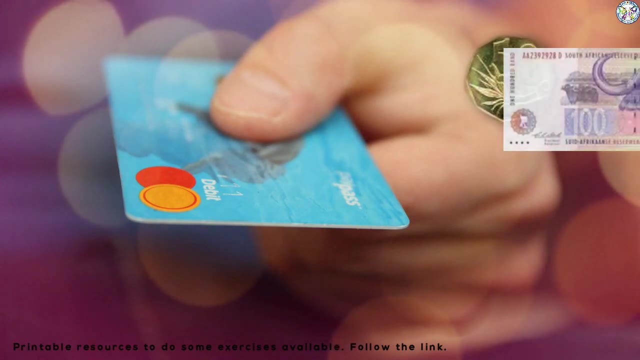 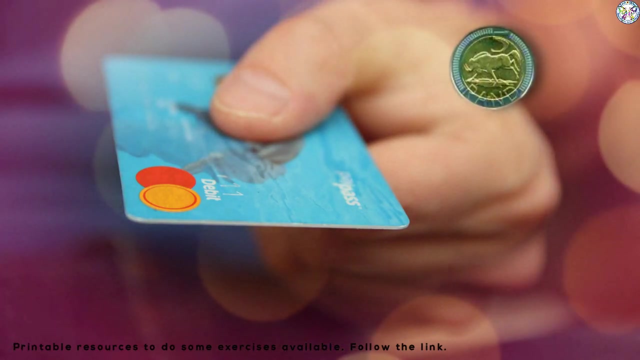 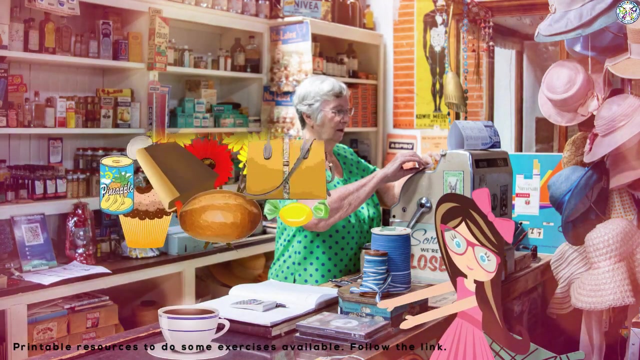 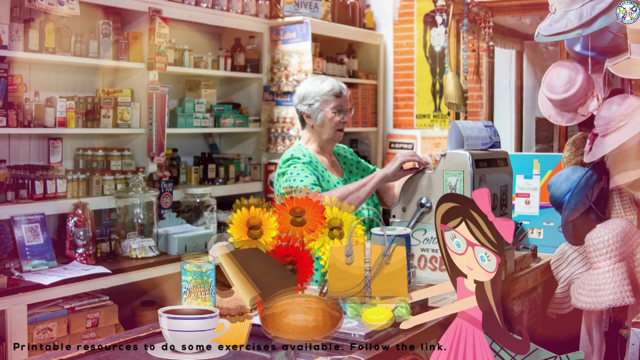 Emma is a bit young to pay with a plastic card. Her parents call it plastic money, That is, a credit or a debit card. She prefers to pay with cash. Emma needs to make sure that she has paid for everything on this day. She goes to the till, where she finds a very friendly lady that will help her to count. 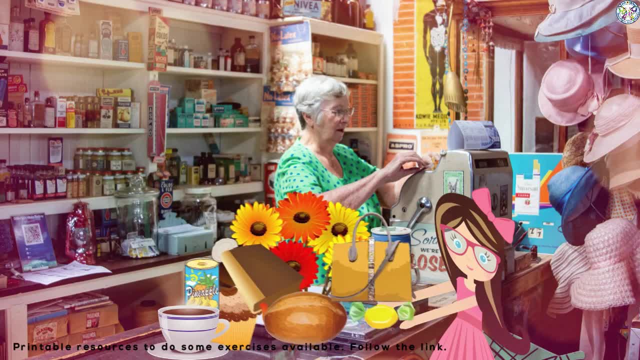 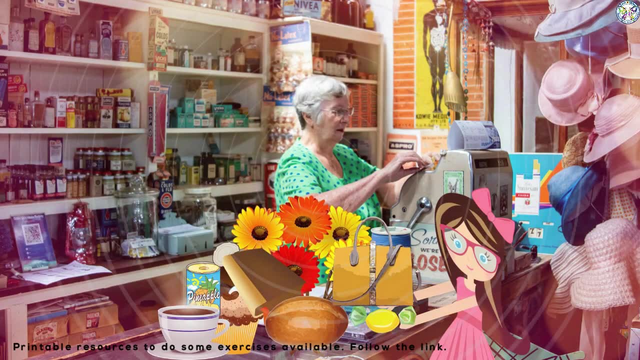 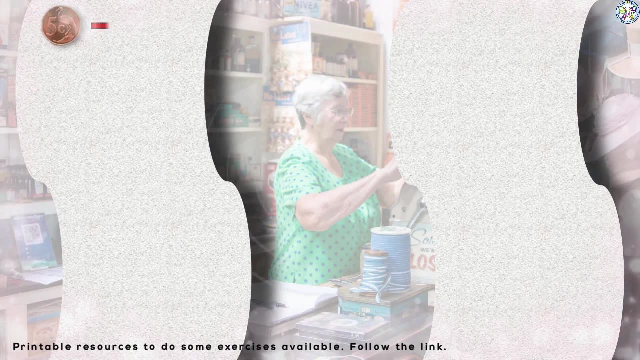 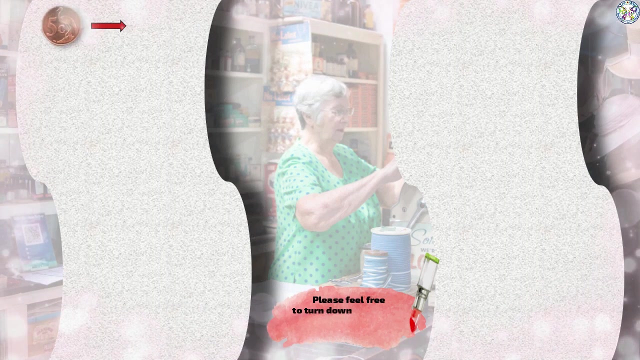 her money and to make sure that she has paid for everything. Let's make sure of the price. Can you remember the price of the items that Emma bought? The five cent she used for buying a sweet, That's right. What did she buy with the ten cent? 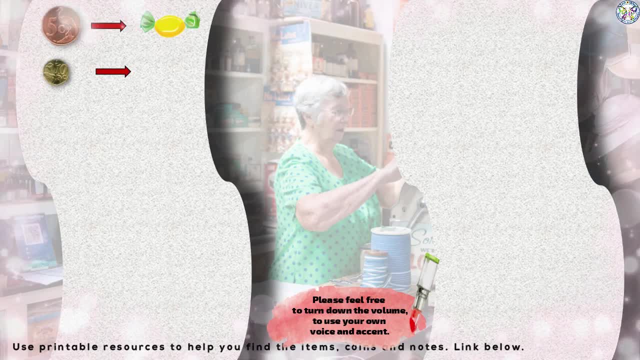 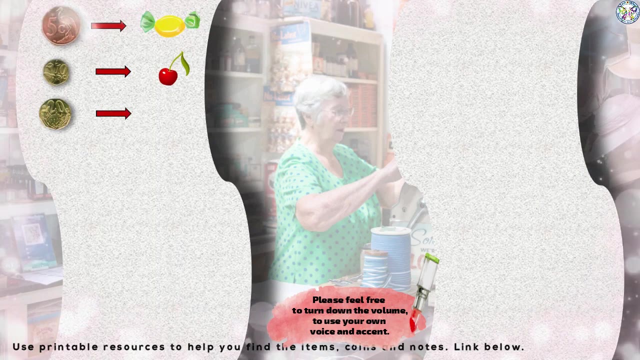 What A cherry. and the twenty cent, The chocolate cupcake. yummy. Fifty cent, Yes. And the bread, Correct, You are doing very well. One rand, The tin of pineapples, Indeed To help her make a hamburger. 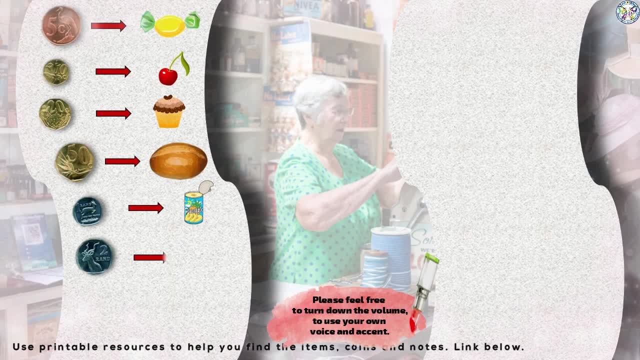 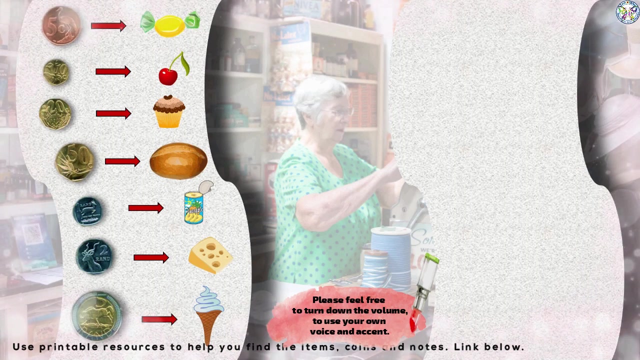 The two rand coin: Yes, Another coin here, A delicious piece of cheese. And the five rand coin- An ice cream. I would also buy it for that price. The ten rand note: Mmm, a nice cup of coffee. The twenty rand note. 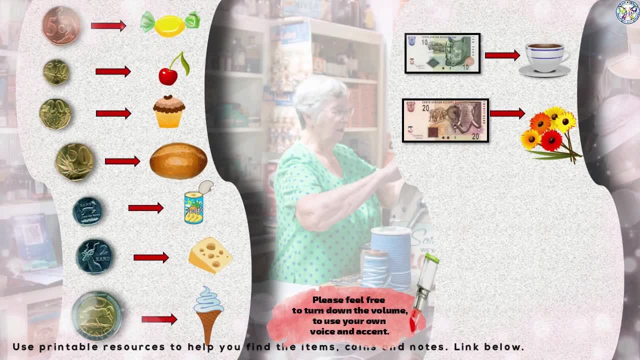 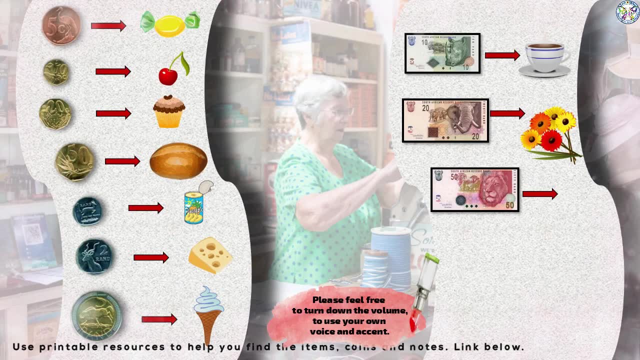 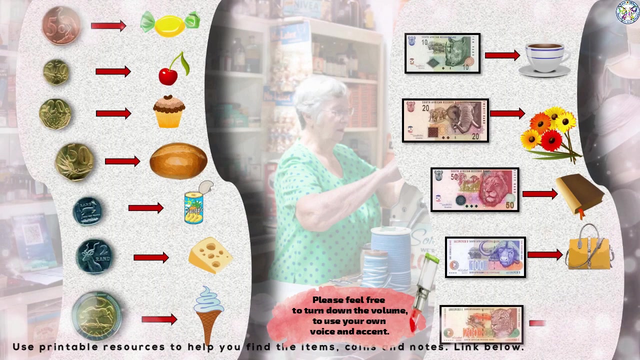 A bunch of flowers for mummy. The fifty rand note: A book, A story book. The hundred rand note: A yellow handbag To keep her money safe. And the two hundred rand note- That's a large amount- A red winter jacket to keep her warm in the days to come. 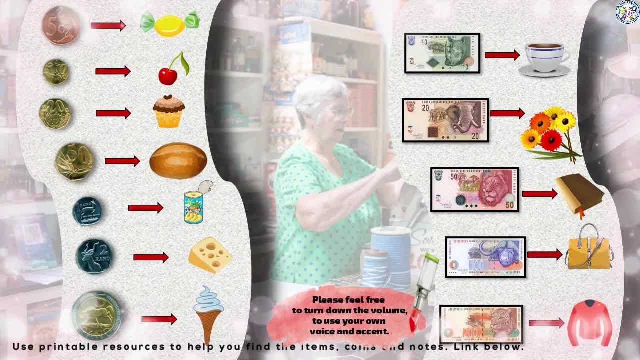 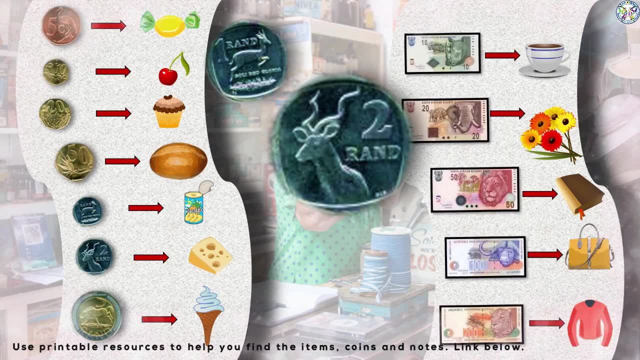 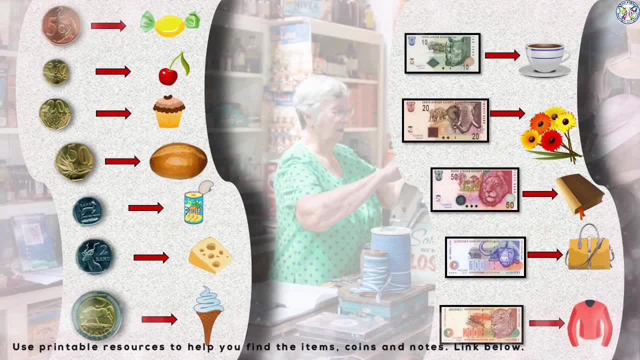 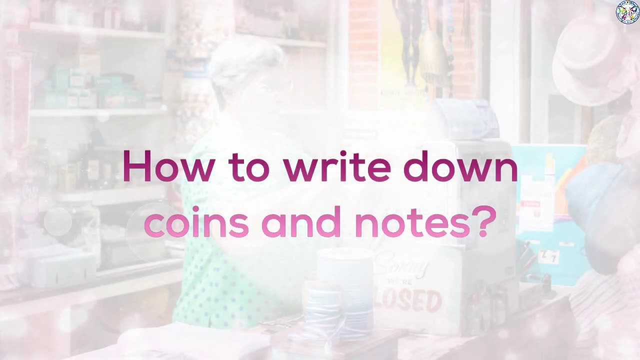 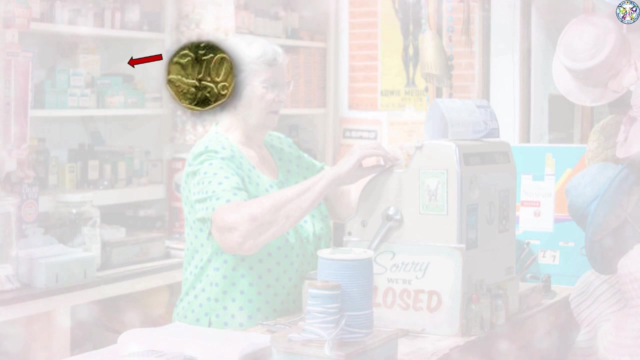 Two rand, Two rand And five rand coins And you know that we have notes. That is paper money. Before we start doing our money sums, let me explain how the coins and the notes work. Here is a ten cent coin. That is one of the coins. 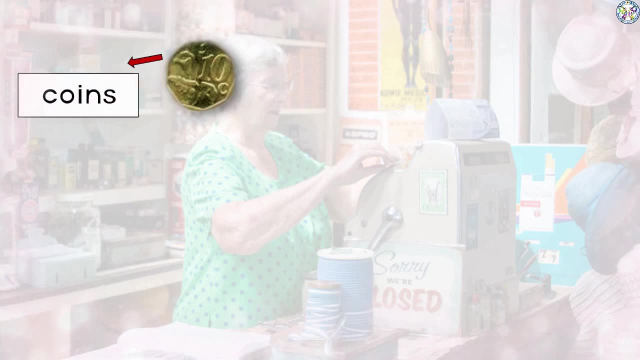 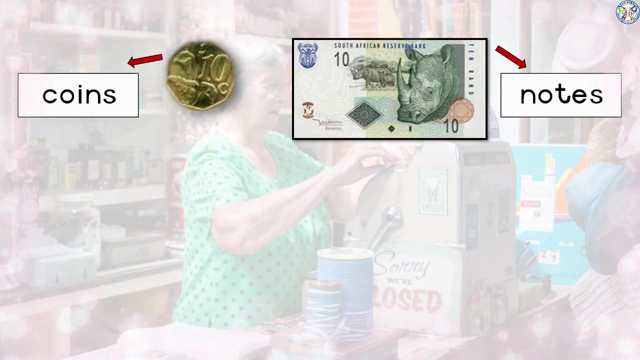 We also have notes, Paper money That they print in the reserve bank. Here is a ten rand note. How do we write down coins and notes? The ten cent We put the k Or the si, Or the si Or the k. 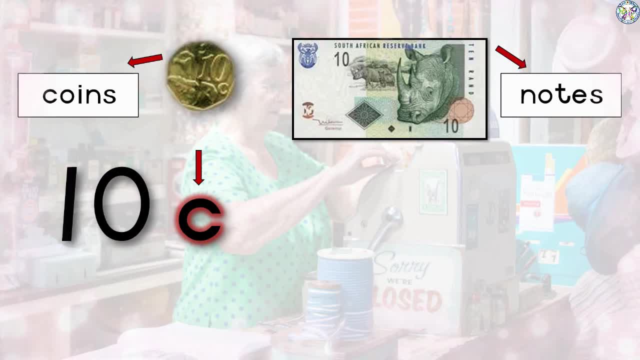 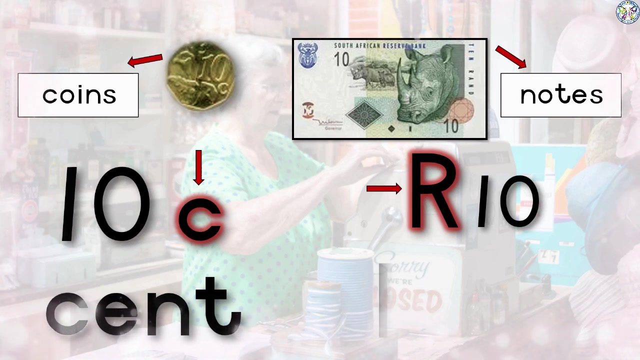 Or the m At the back of the number. Can you see that? And the notes we put the R or the R, capital letter in front of the number. K or C stands for cent at the back of the number And the R or the R stands for rand in front of the number. 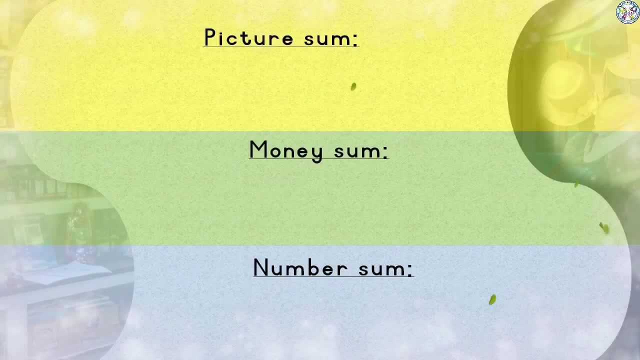 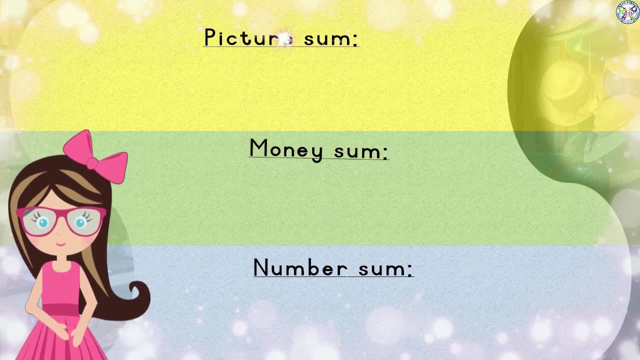 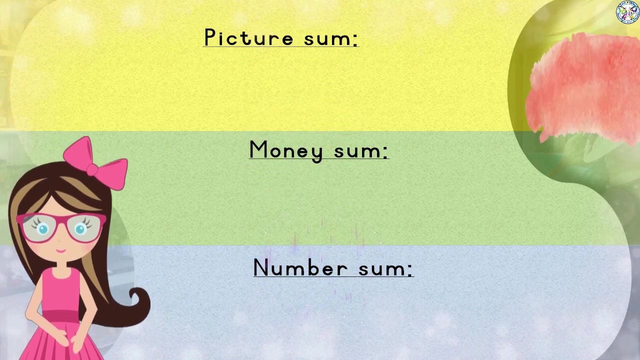 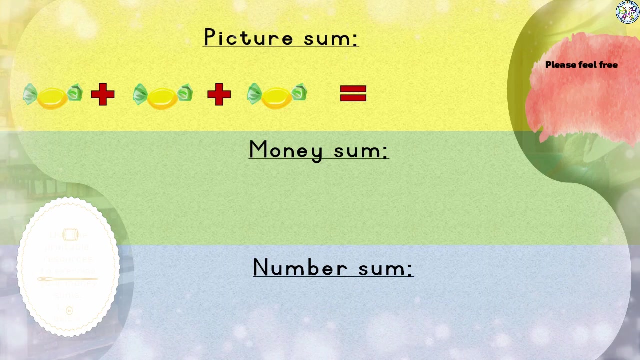 Now that you know how to write down money, let's build a couple of money sums. We have a picture sum, money sum and a number sum. Let's explain: One sweet plus one sweet plus one sweet gives three sweets. Can you see that Easy? Let's build a money sum. 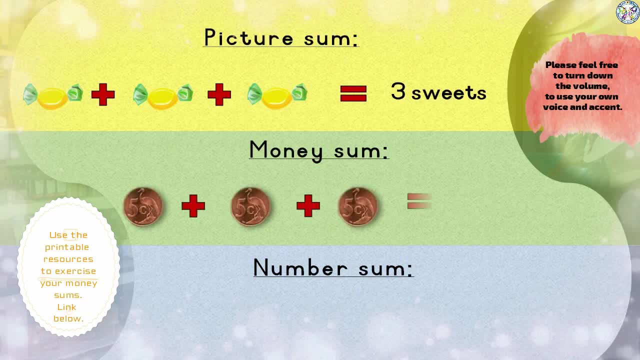 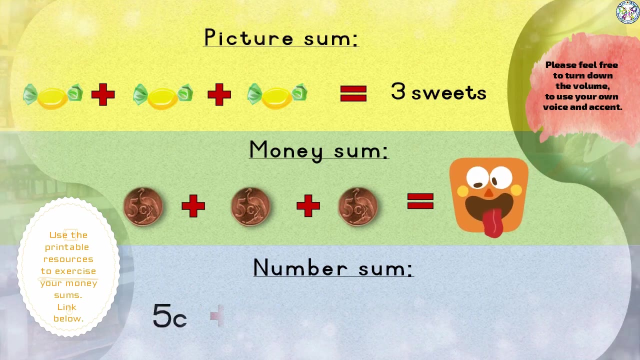 Five cent Plus five cent plus five cent. Can you count in fives Easy, It makes up fifteen cent. And now for the number sum Five cent plus five cent plus five cent. The answer you've worked out already. 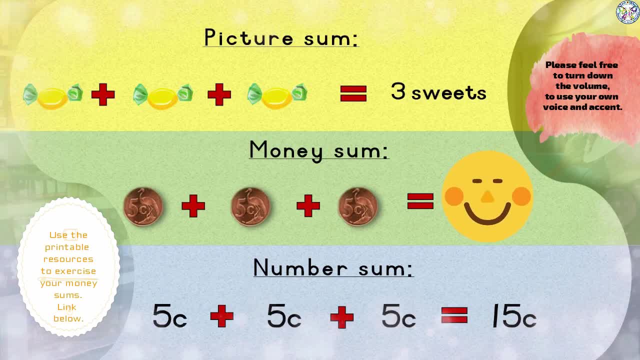 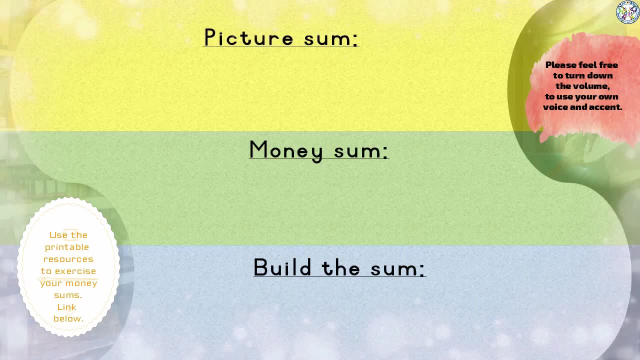 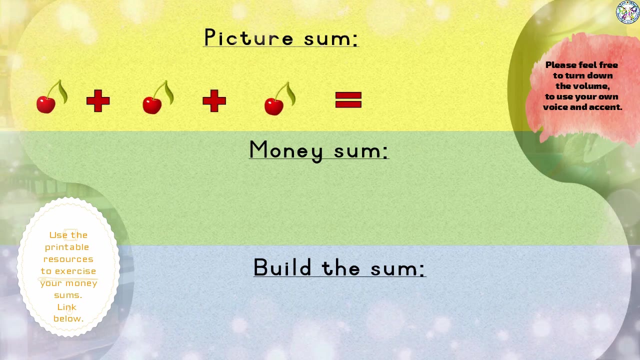 Fifteen cent. Easy as pie, Let's do another one. The picture sum Cherry plus a cherry plus a cherry gives me three cherries. Now for the money sum Ten cent plus ten cent plus ten cent. 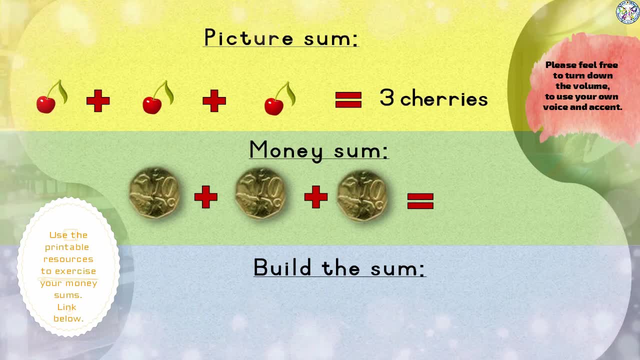 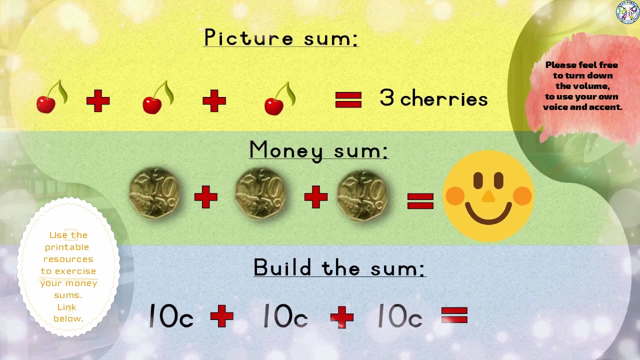 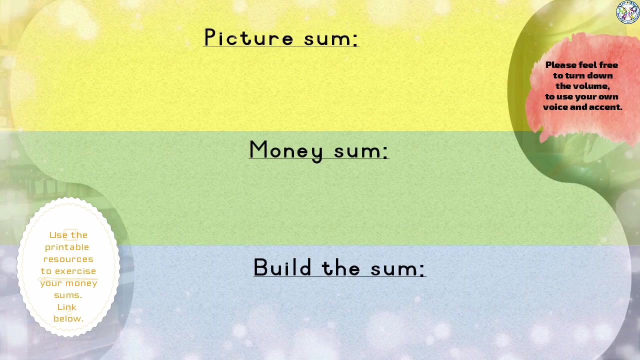 Count in tens, Thirty cent. Now let's build the sum, Write down the numbers: Ten cent plus ten cent plus ten cent. It gives me- Do you know the answer? Thirty cents. Well done, Are you ready, Ready for a couple more? 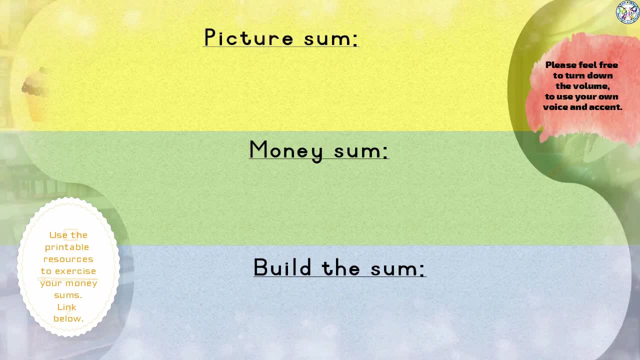 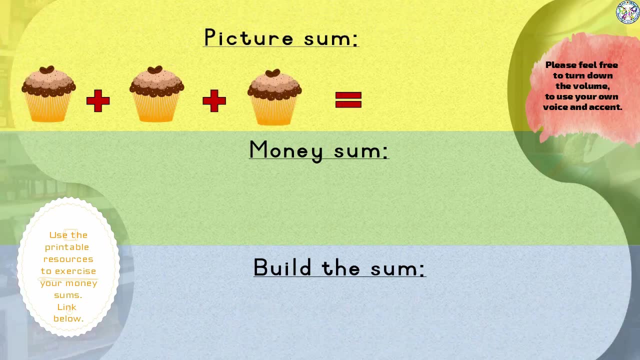 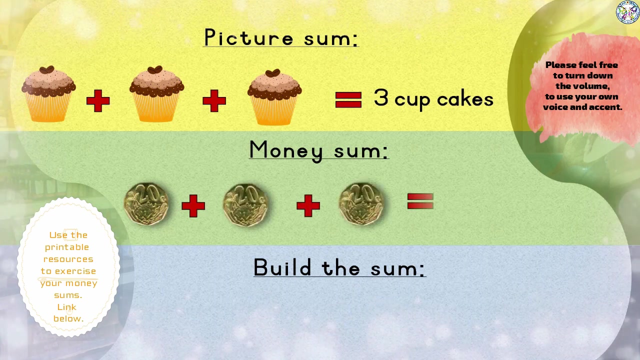 Picture: sum Cupcake plus another cupcake. plus another cupcake gives me Three cupcakes indeed. Twenty cent plus twenty cent plus twenty cent, Twenty cent, up a total of: Can you count in twos, It's almost the same. Sixty cents, Build the sum. 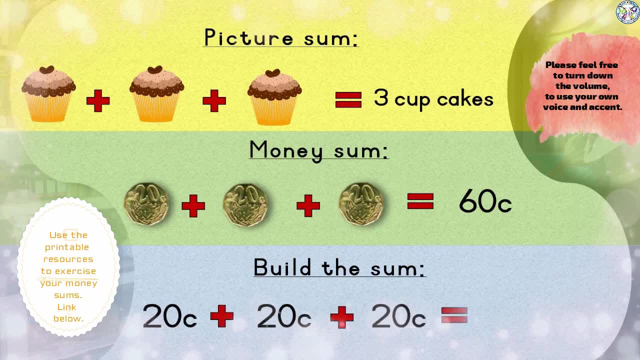 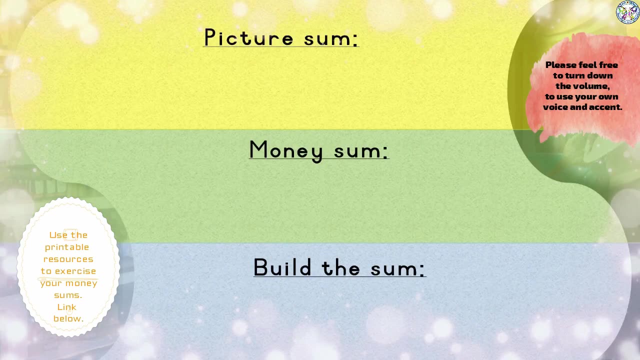 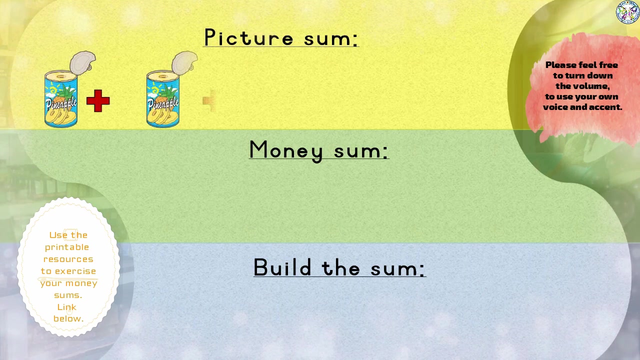 Twenty cent plus twenty cent plus twenty cent makes up. Do you know the answer? Sixty cent. You're doing quite well. Ready for more Picture: sum One tin plus another tin plus another tin gives me, That's so easy, Three tins. Let's build the money. sum One rand. 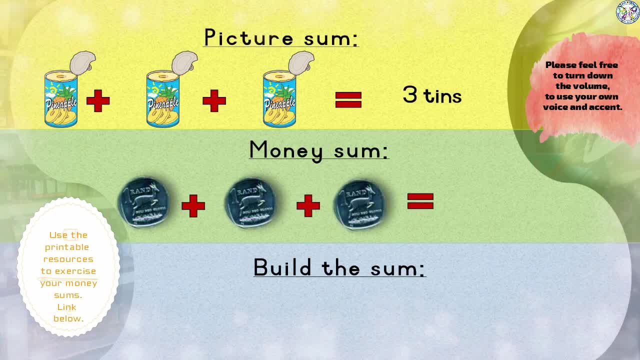 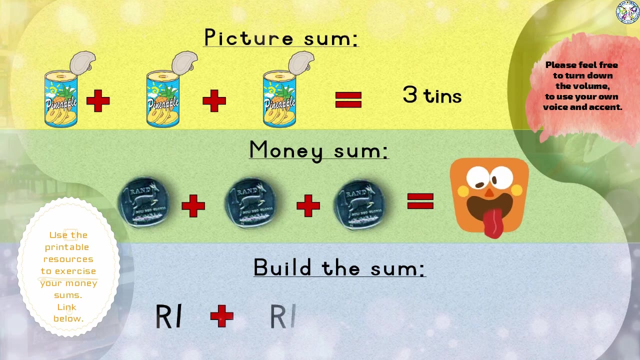 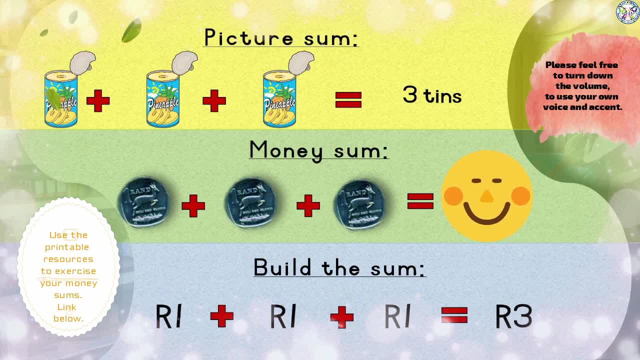 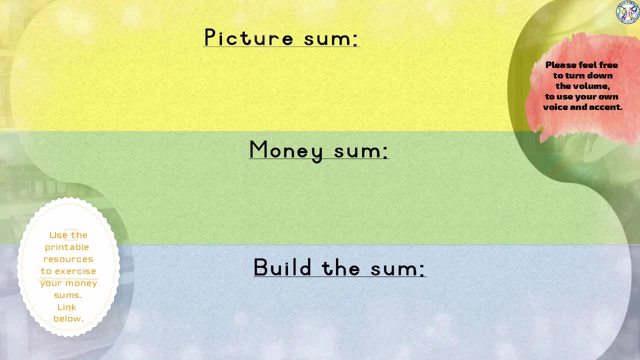 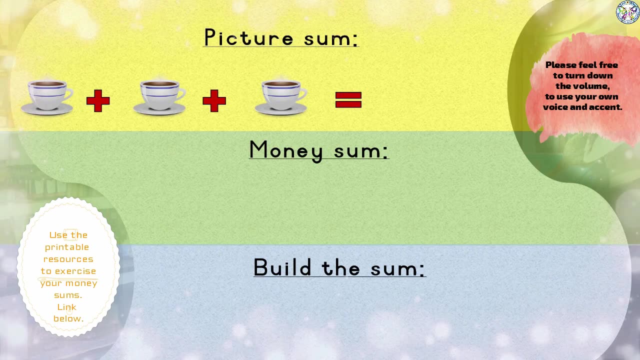 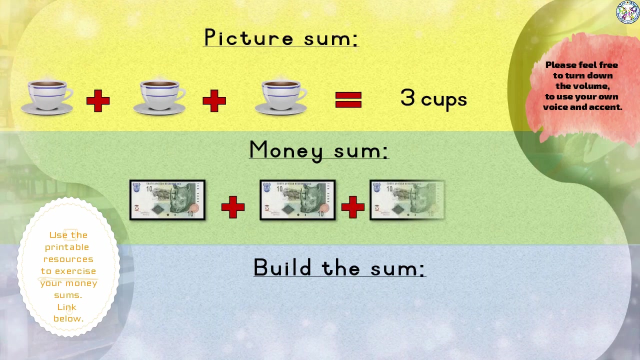 Ready for more. It's getting easier, don't you think? Picture: sum: A cup of coffee plus another cup plus another cup. It gives me Three cups. Let's use our notes: Ten rand plus ten rand plus ten rand. It gives me Just count in tens. Easy Thirty rand. Replace the notes with numbers. Ten rand. 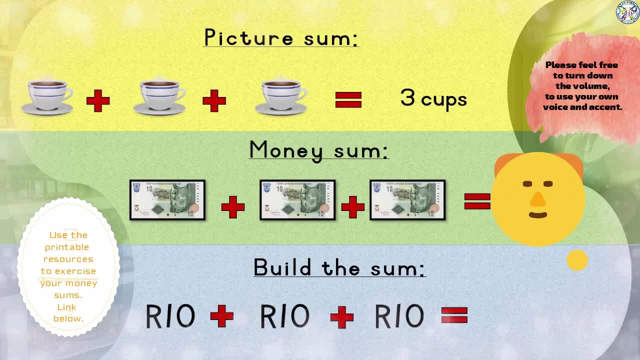 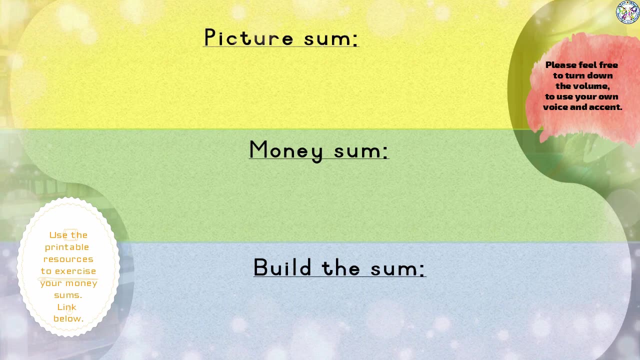 plus ten rand plus ten rand, It gives me, Can you remember, Thirty rand investigación. One rand plus one rand plus one rand plus one rand Two. Yes, I'm one rando, Three per cran pounds. One rand, One ru, Two rand, Which rand? 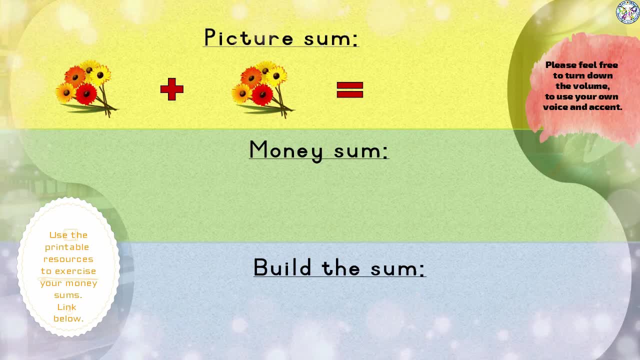 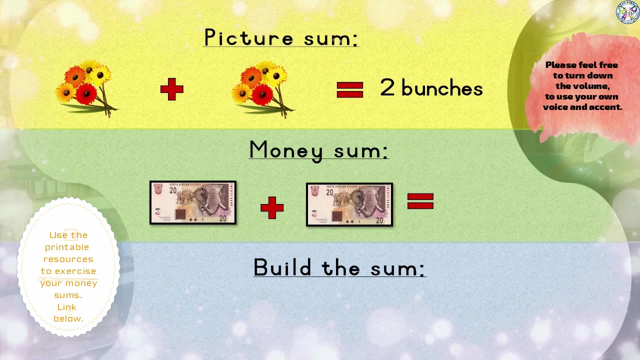 One ru Aعد. Last one, The είena is made up of cenu Fue chah invalidate. Then we can write it down. Thank you for watching today. banj on twitter. on instagram, counting twos. 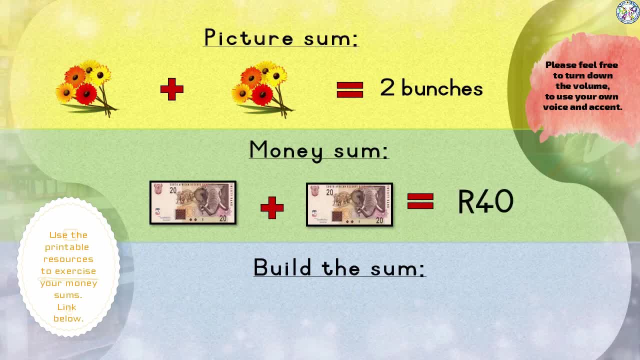 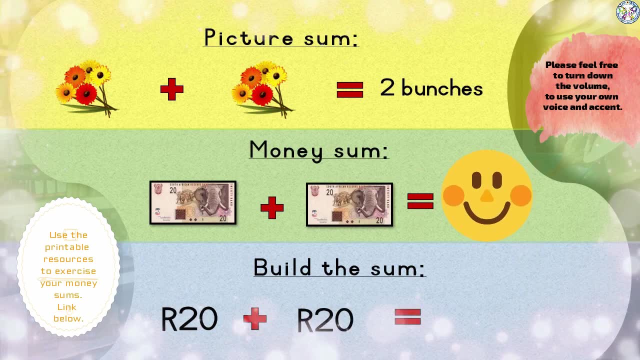 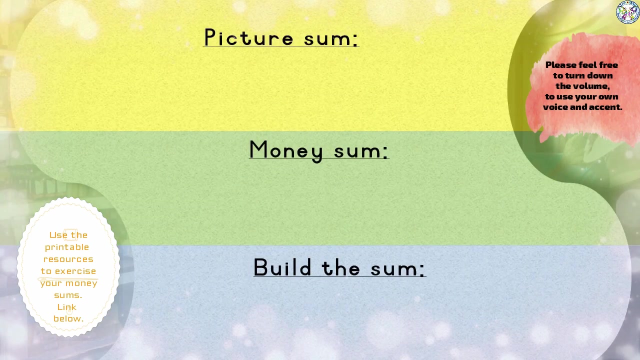 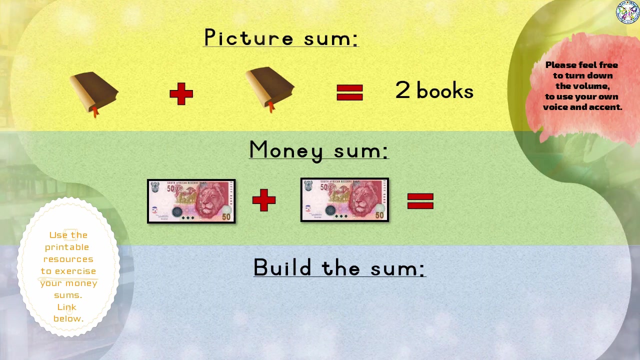 forty rand. replace the notes with numbers. twenty rand plus twenty rand, max up forty rand. well done, a book plus another book gives me two books. quite right, easy. let's do the money sum. fifty rand plus another fifty rand will make up hundred rand. let's replace the notes with numbers. 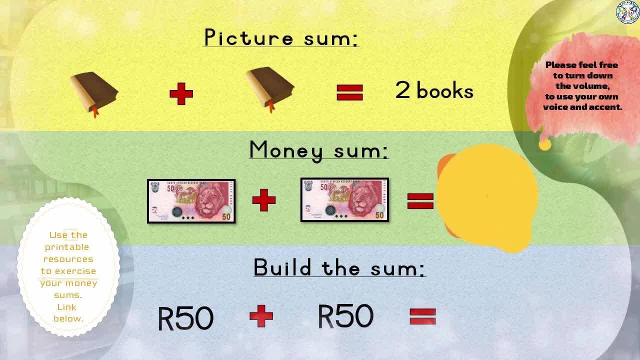 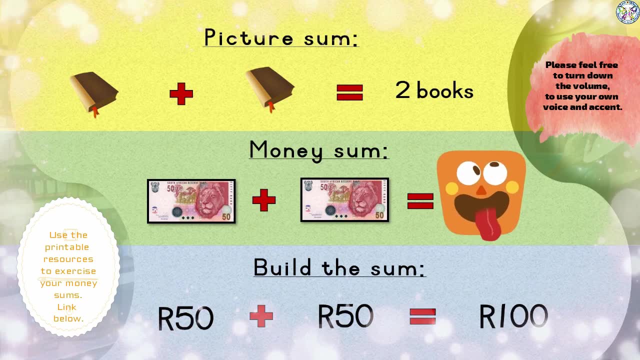 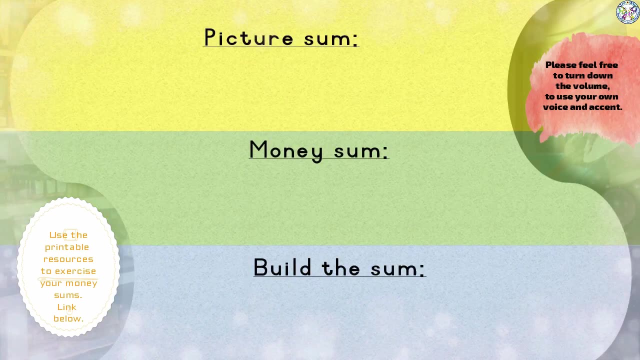 fifty rand. add another fifty rand equals hundred rand plus another hundred rand will make up a hundred rand. well done, the last one before we mix up, putting together our cents and rands. one handbag plus another handbag gives me two handbags. let's do the money sum. 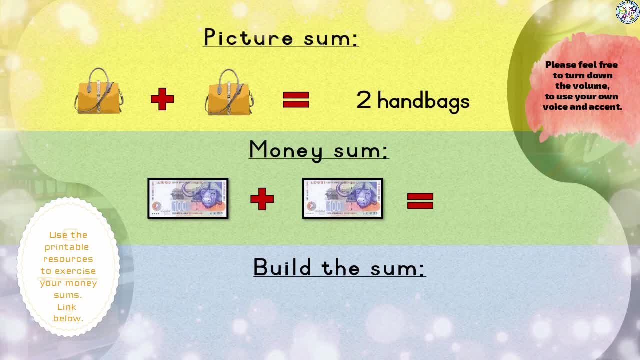 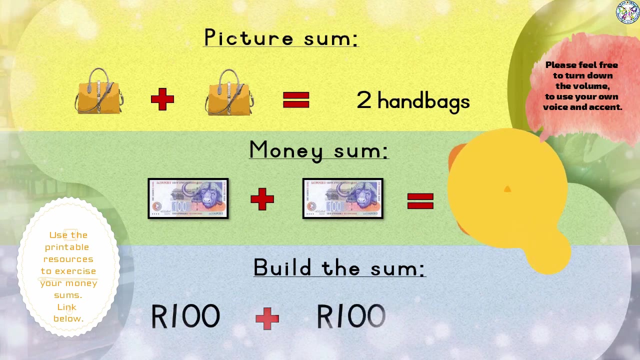 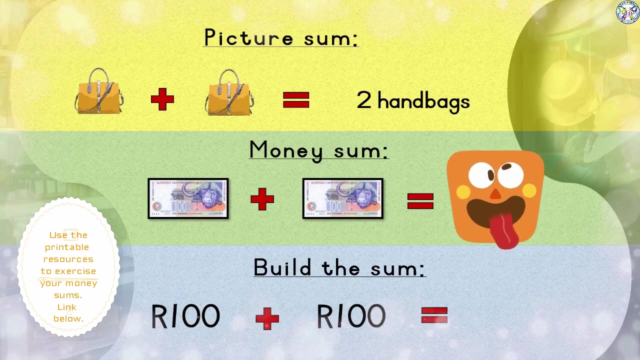 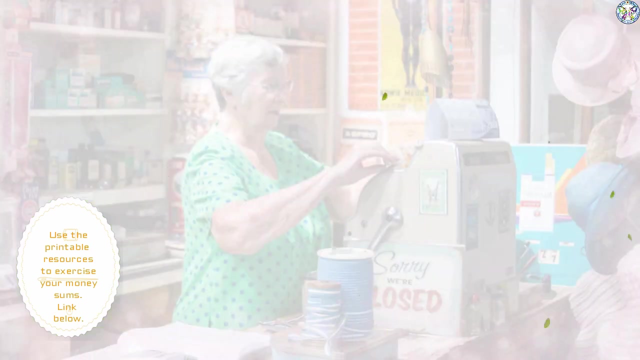 hundred rand, Two hundred rand. Always write the R in front of the number. One hundred rand plus one hundred rand will make up two hundred rand. How to write down combinations between cent and rand. We have coins, but you remember, not all coins are cents. 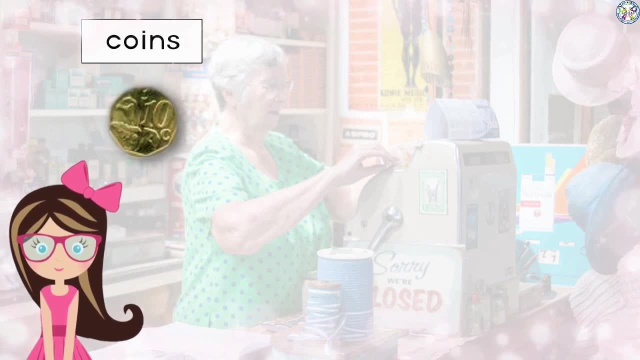 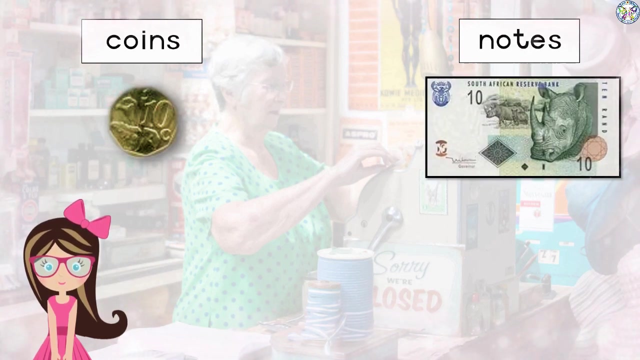 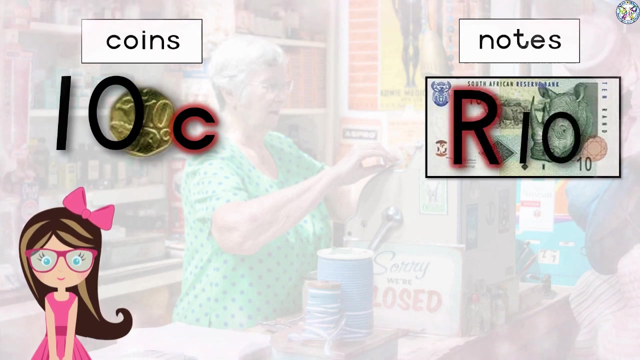 Let's take the ten cent for an example Notes. Here is the ten rand note: This is ten c for cent And the ten rand the R in the beginning of the number, always in a capital letter. Now we want to put them together plus. 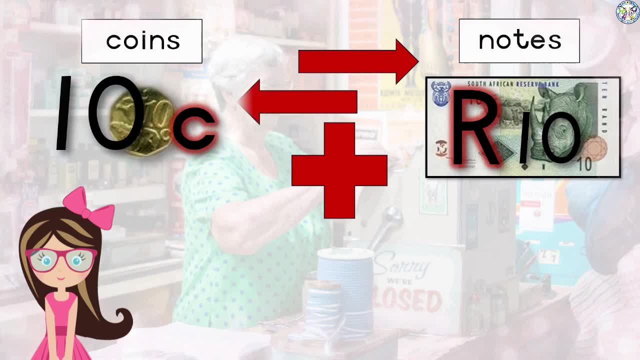 Always use the bigger note and then the smaller coin. You put them together: The biggest one first, Ten rand, Followed by the smaller coin, The ten c for cent. But how to make sure that you understand that there are rands and cents? 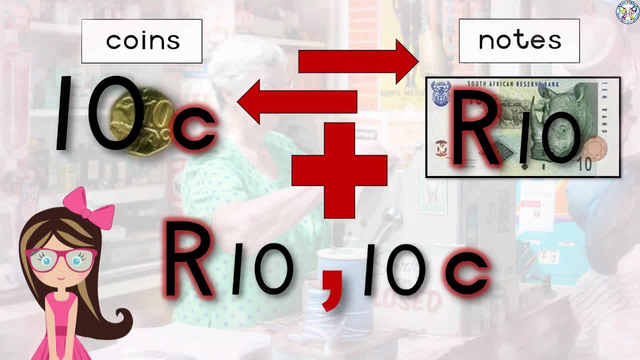 You will have to put a placeholder, A comma in between the rands and cents And a comma in between the rands and cents. And you know what, If you do this, you don't always have to write down the c for cent. 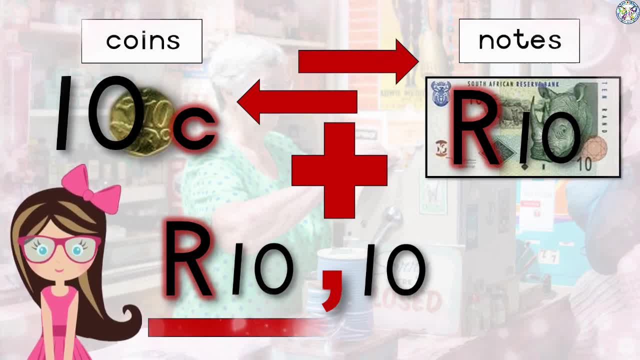 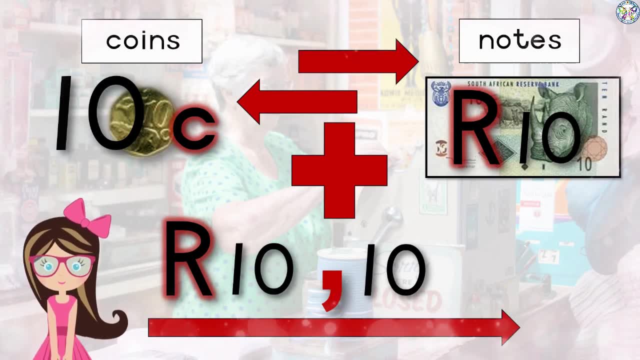 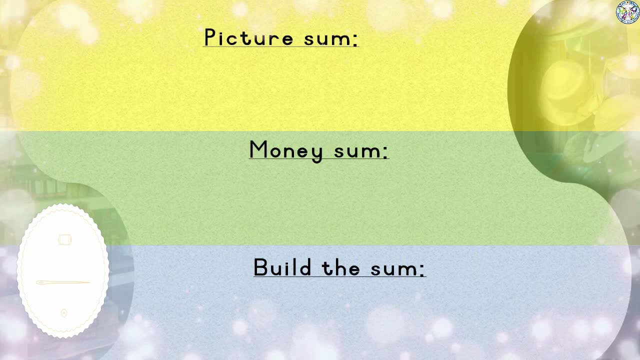 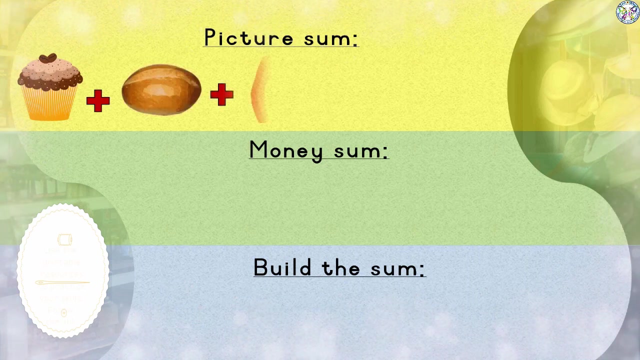 Ten rand, comma ten cents. Good, Let's do some combination sums where we put together the rand and the cents. Picture sum: One cupcake Plus a bread roll Plus a jacket Will give me. I can't add that up. 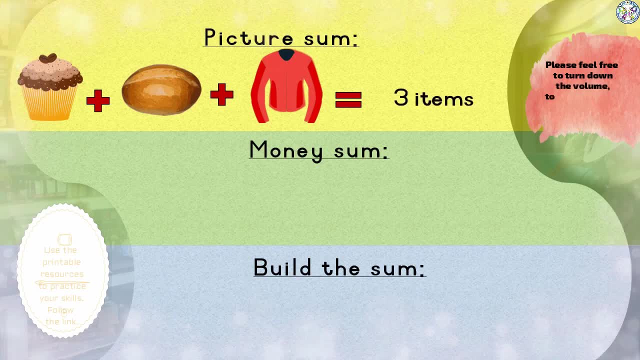 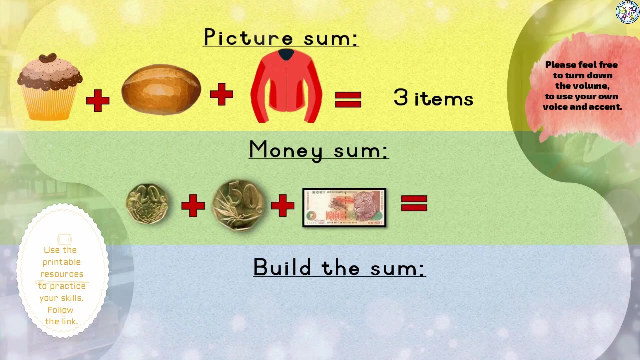 So I just write down Three items Now for the money sum: Twenty cent Plus fifty cent Plus two hundred rand. If we add it up It will make up. Remember the biggest one, first, Two hundred rand, comma seventy cents. 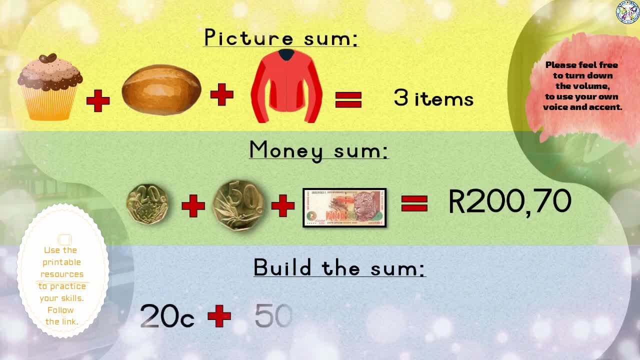 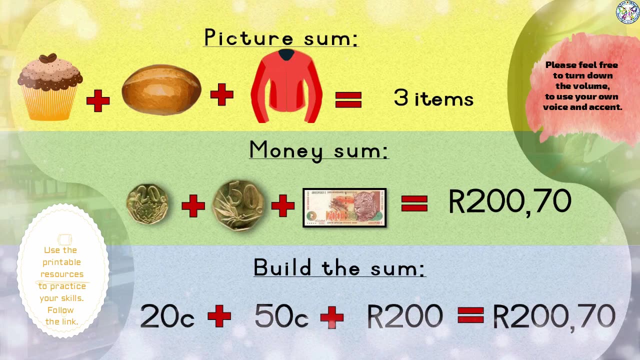 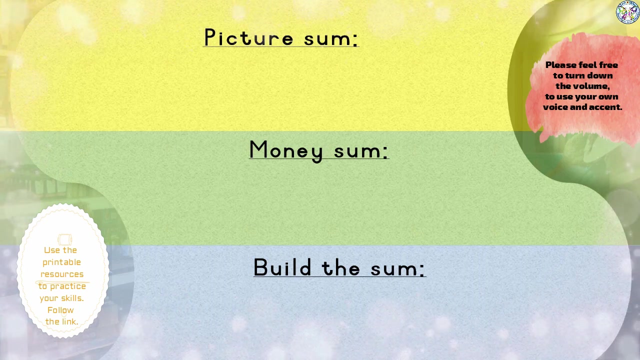 You don't need to write down the c for cent. Twenty cent plus fifty cent plus two hundred rand. Think You know the answer: Two hundred rand, comma. seventy cents. Seventy cents. Well done, Let's try another one: An ice cream plus a cup of coffee, plus another cup of coffee. 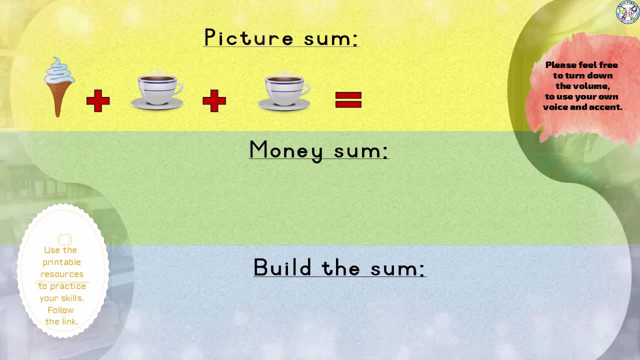 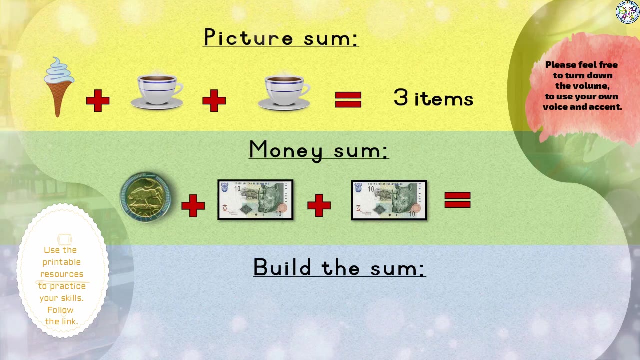 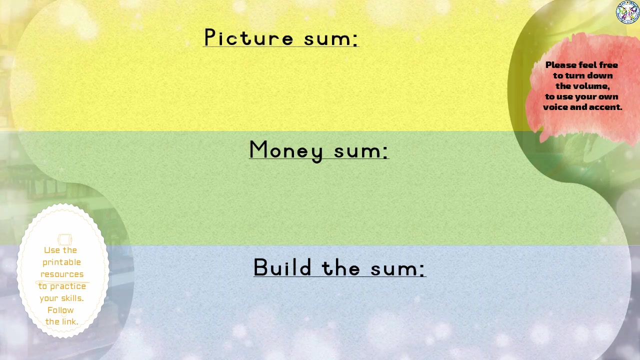 Will give me Three items Now for the money sum: Five rand plus ten rand plus another ten rand plus another 10 rand. add it up: 25 rand, 5 rand plus 10 rand plus another 10 rand. if we add that up 25 rand, well done, picture some: a cherry plus a cupcake. 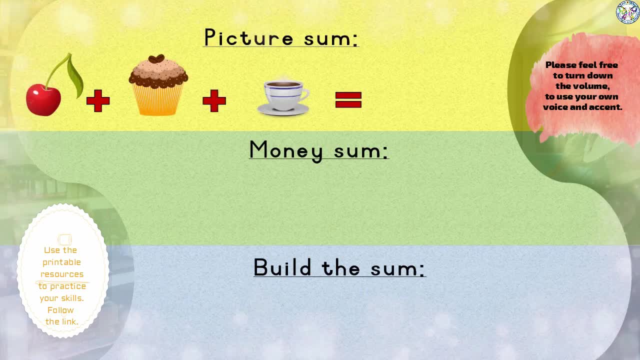 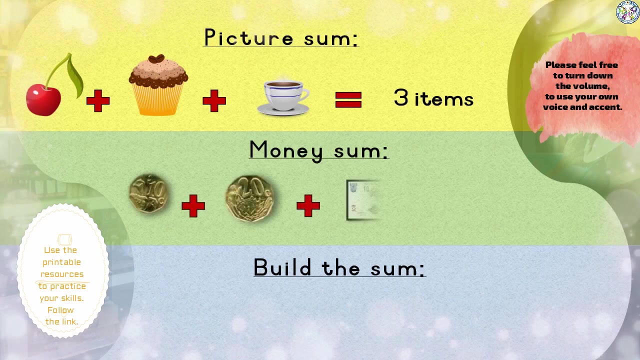 plus a cup of coffee. three items: 10 cent plus 20 cent plus a tin round. note: add it up: 10 rand comma 30 cents. build the some 10 cent plus 20 cent plus another ten rand plus 20 cent plus 10 rand. 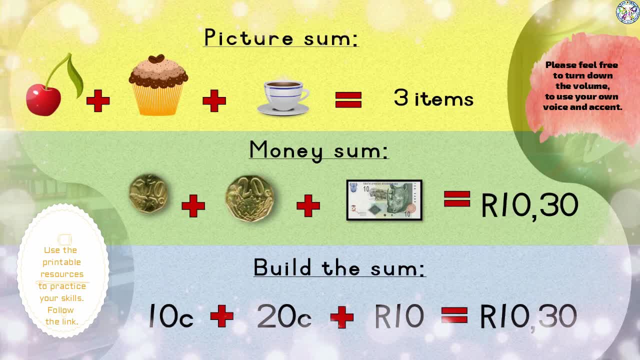 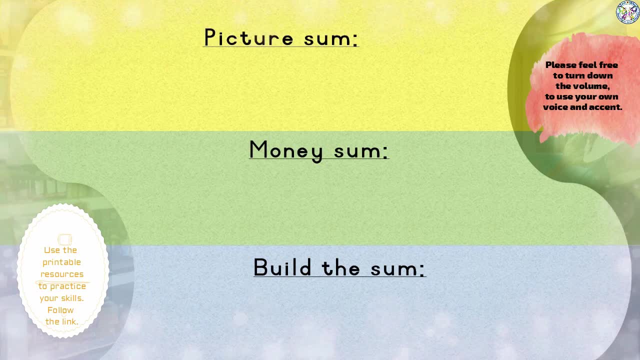 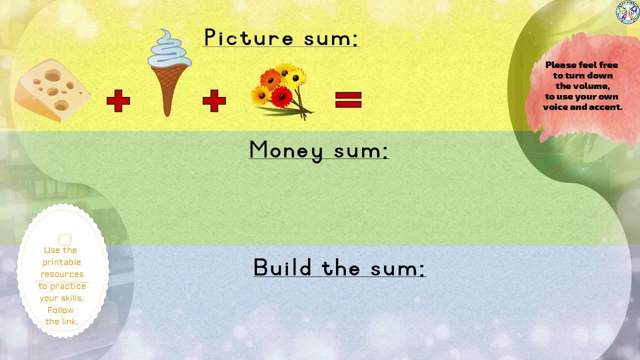 10 rand comma 30 cent. Let's do the last one before we go to the shelves to pick the products ourselves. Cheese plus ice cream plus a bunch of flowers: It equals three items. Now for the money sum. 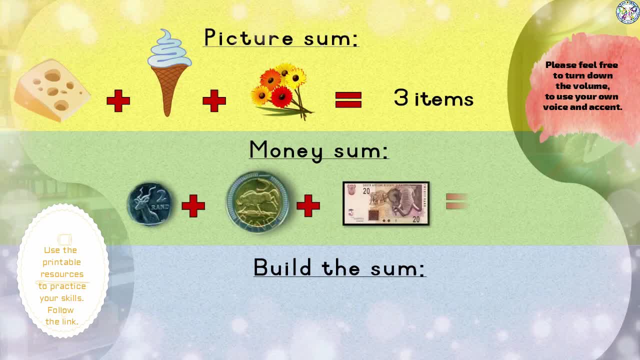 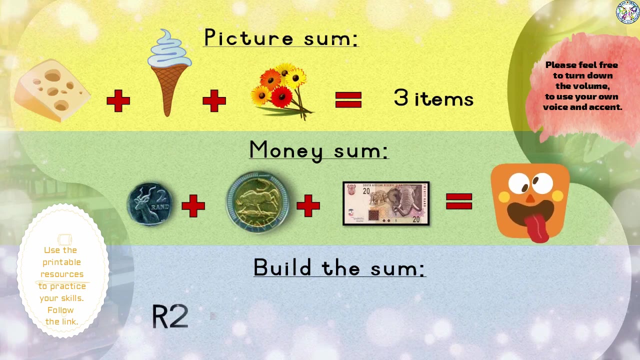 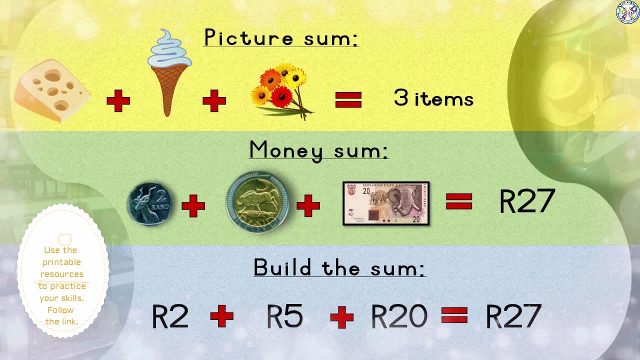 2 rand plus 5 rand plus 20 rand. Mix up 27 rand. correct Build the sum 2 rand plus 5 rand plus 20 rand Equals 27 rand. Let's go to the shops to pick out the items on the shelf. 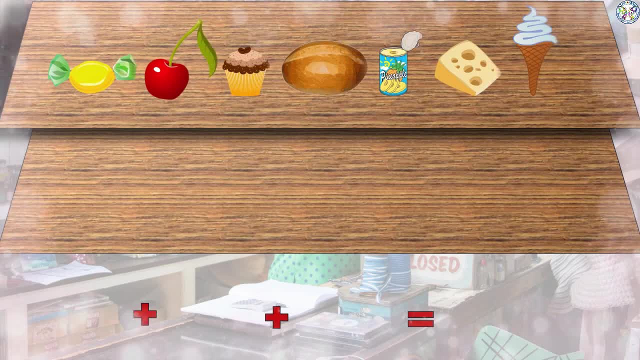 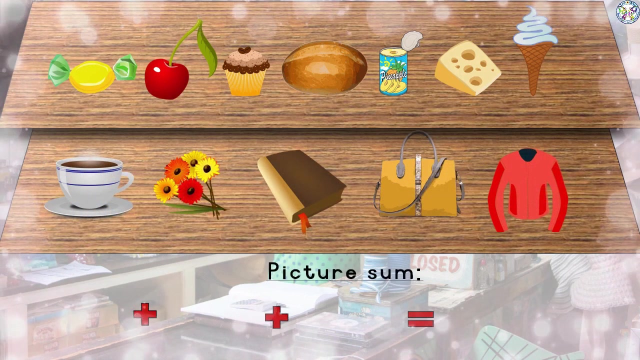 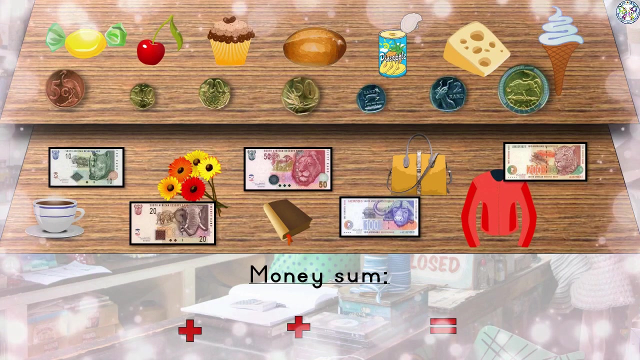 Top shelf items. Let's do a picture sum: Bottom shelf items- Bottom shelf items- Bottom shelf items- Top shelf items. An ice cream and a cherry to put on top of the ice cream, and that equals 3 items. Let's replace the items with the money value, a money sum: 2 rand plus 5 rand for the ice. 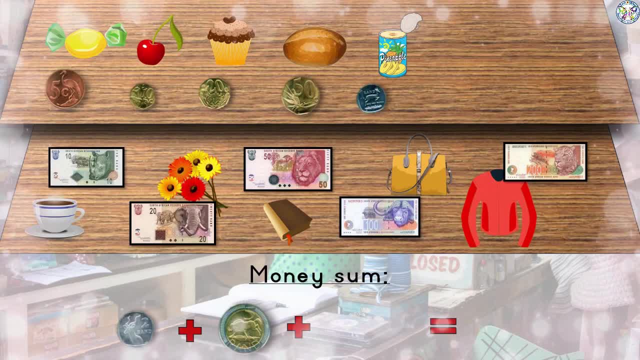 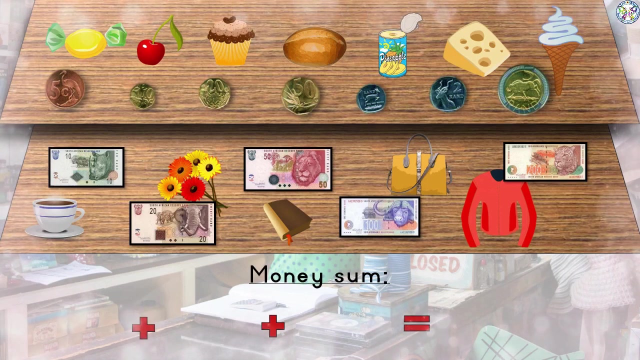 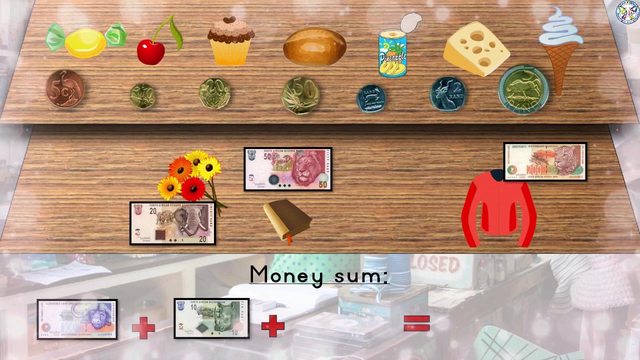 cream plus 10 cent for the cherry. Add it all up and it will give me 7 rand and 10 cents- good Money sum handbag for 100 rand cup of coffee: 10 rand And 50 cents. add it all up: 110 rand and 50 cents. 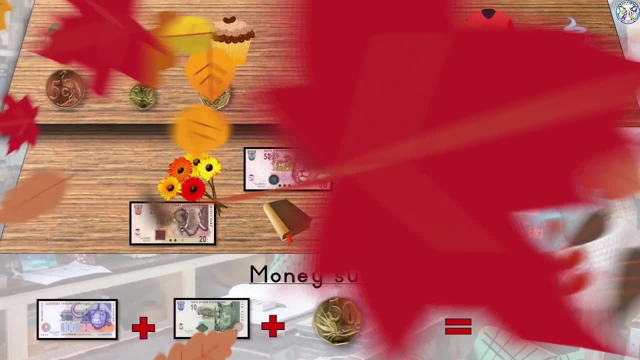 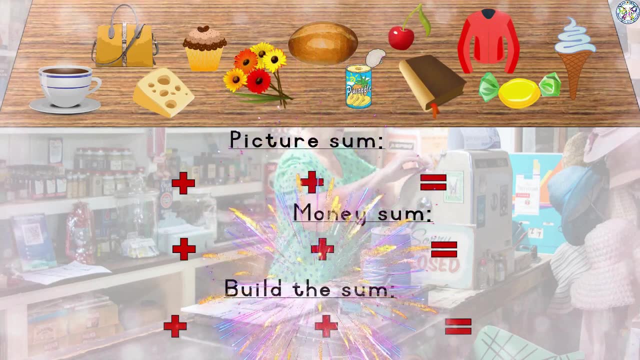 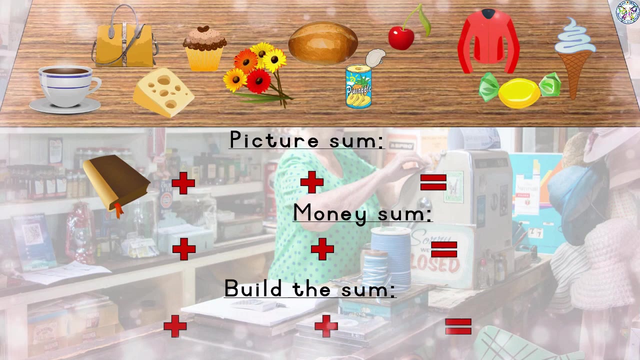 Well done, let's sum it all up. We have picture sum, money sum And then we can sum it all up. We can build the sum replacing the coins or the notes with numbers: a book plus a cup of coffee plus a chocolate cupcake. 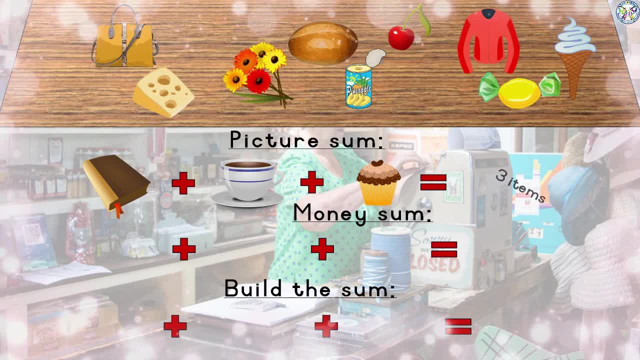 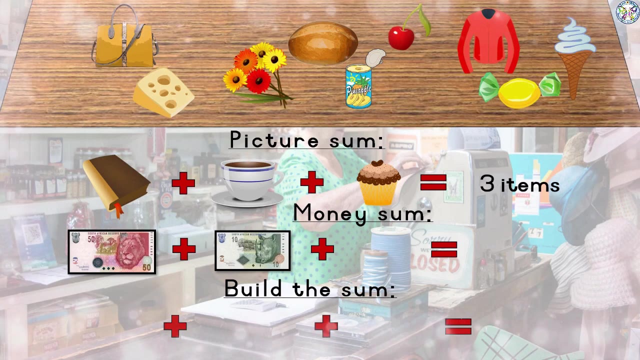 Equals, you know it by now- 3 items. So it is 50 rand plus a 10 rand note plus a 20 cent coin. Add it all up and it will equal 10 rand, And then we can sum it all up. 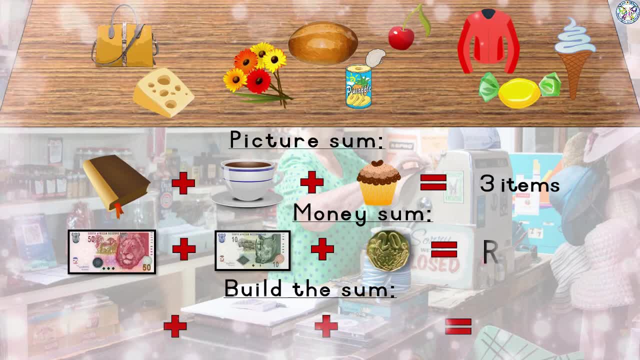 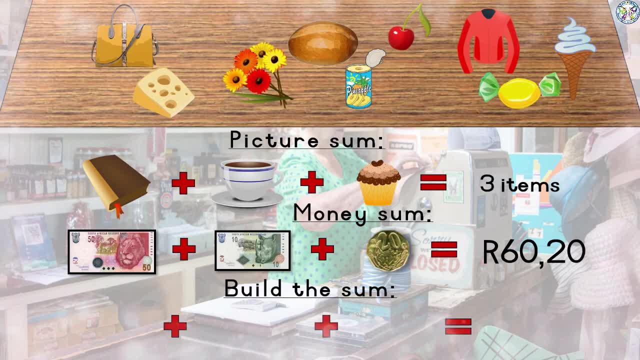 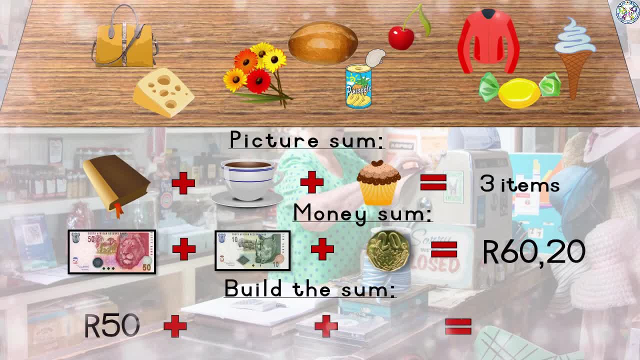 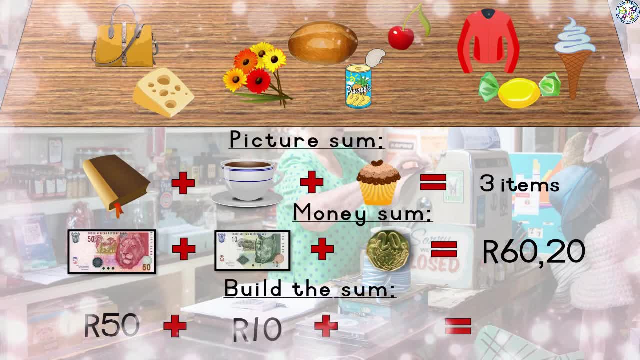 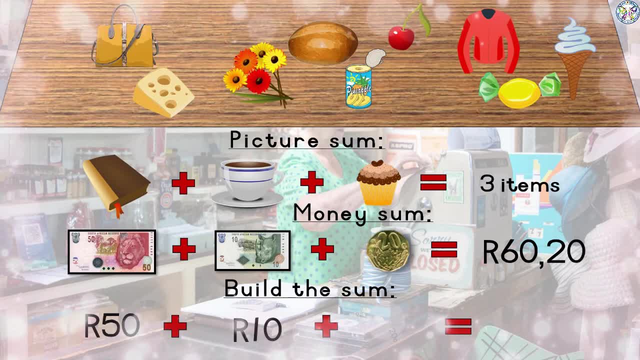